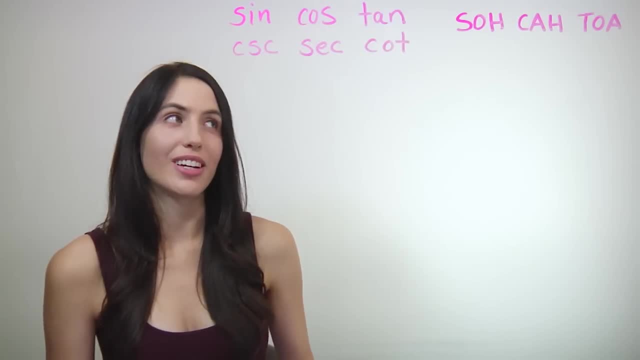 cosine and tangent, And we're going to use the memory trick SO-CO-TOA, which a lot of people say quickly as SO-CO-TOA, But this is what it is, It's a memory trick to remember what sine, cosine and tangent mean. So we'll use that. All of these six trig functions. 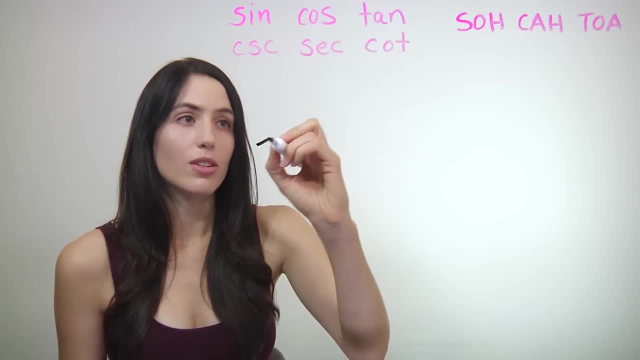 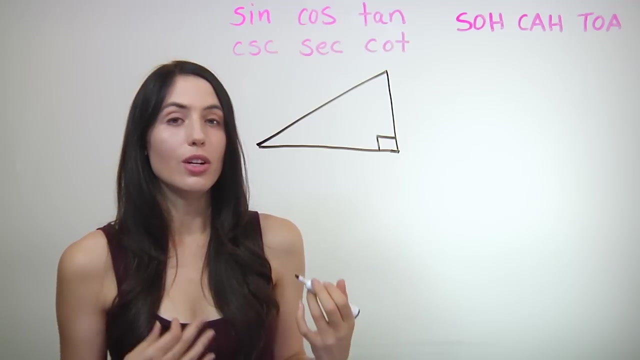 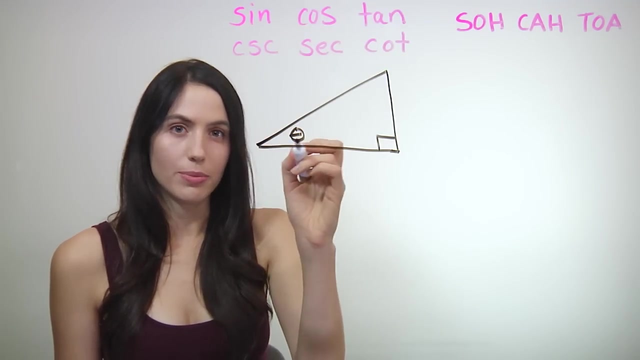 involve right triangles. That is, a triangle that has a right angle in the corner, which is noted by the corner symbol down here. So it's 90 degrees, a right angle, And you can also know where theta is. It will be labeled on your triangle. Theta is just an angle. 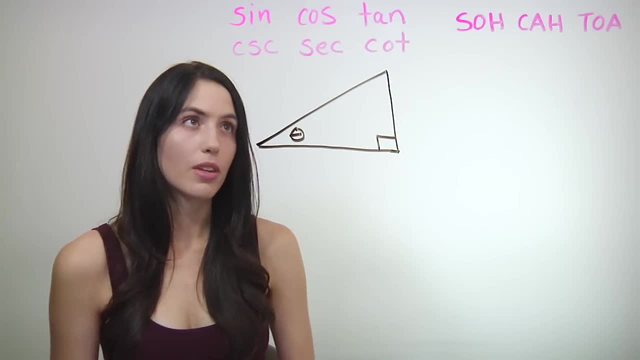 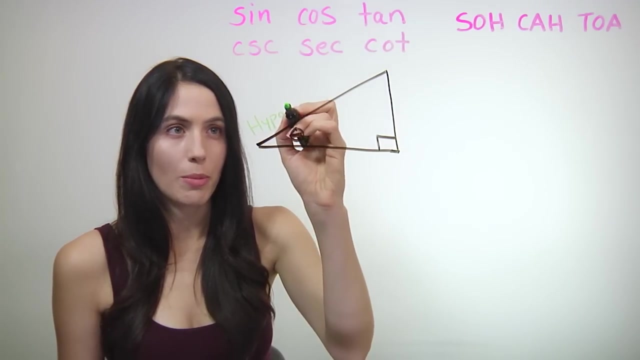 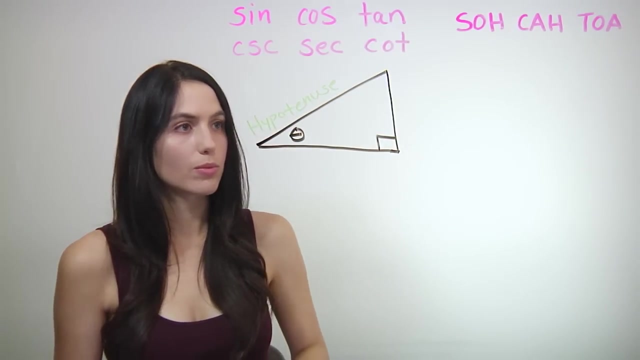 It's an angle that is not your right angle. What's important to know is what each of the sides of the triangle are in relation to theta. What I mean by that is, the longest side on the triangle is called the hypotenuse, So you'll just want to remember that the longest side is the hypotenuse. The other side that 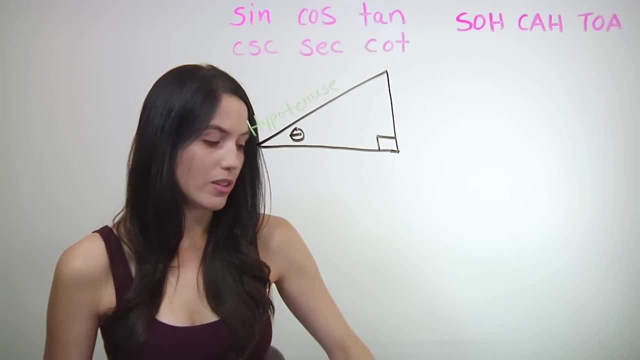 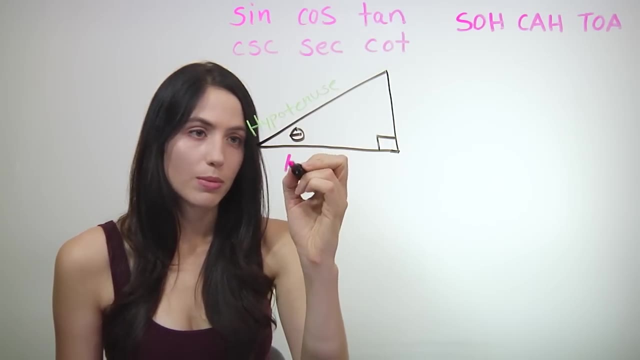 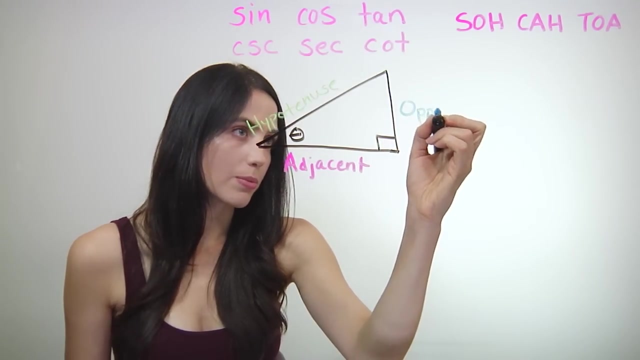 is next to theta. that is not the hypotenuse- is called the adjacent side. It's adjacent to theta, but it's not the hypotenuse. And the other side, the third side, is the adjacent side. The hypotenuse is opposite theta, directly opposite theta, and it's the opposite side. 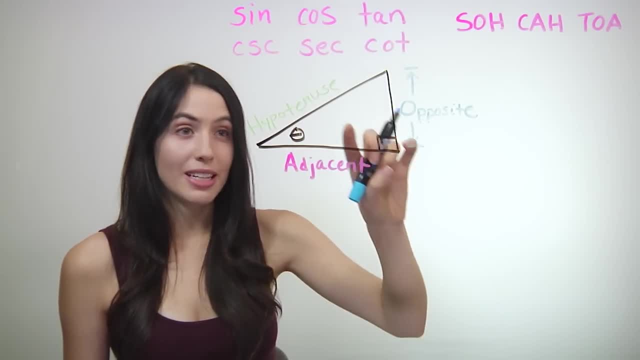 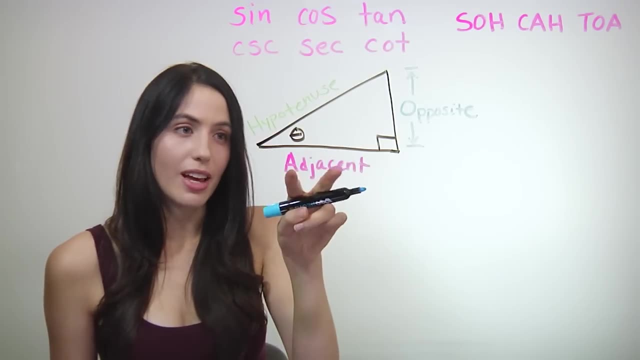 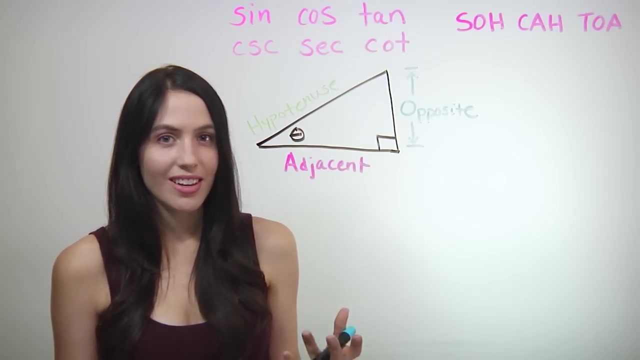 So notice that the hypotenuse is immediately opposite the right angle, The opposite side is opposite theta and then the adjacent side is the other side next to theta, that is not the hypotenuse. So you will use those to evaluate sine cosine and tangent. 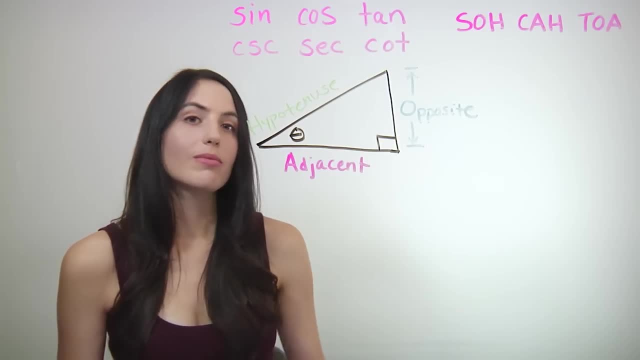 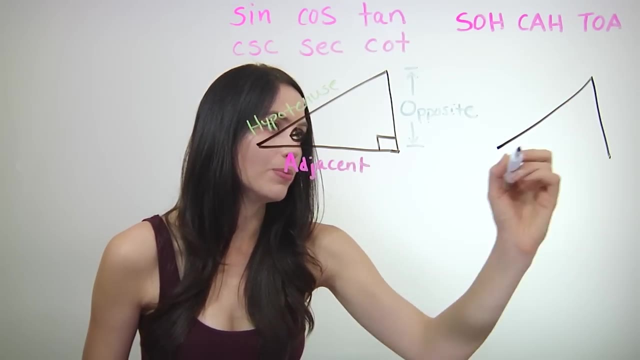 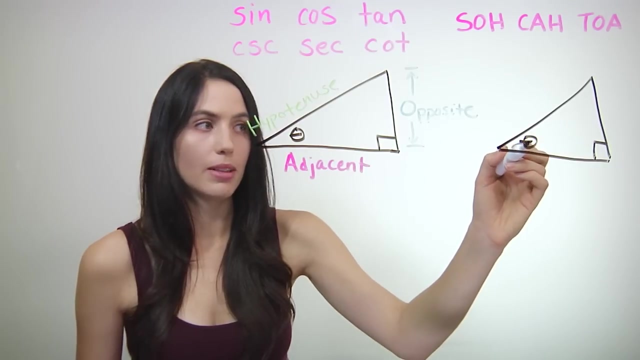 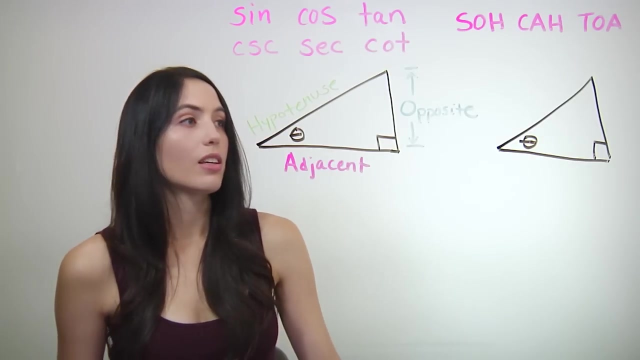 So you might be working on a problem that looks something like this where you're given triangle, you write triangle, the right angle, some theta labeled on your diagram and then side lengths that are given to you. So, for instance, you might be given that the longest. 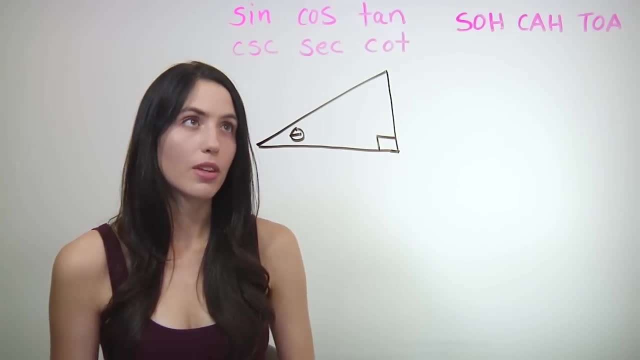 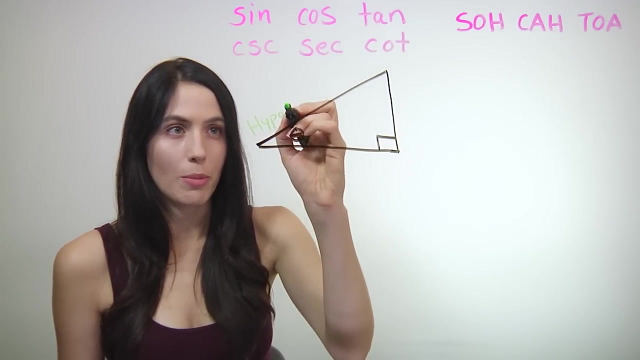 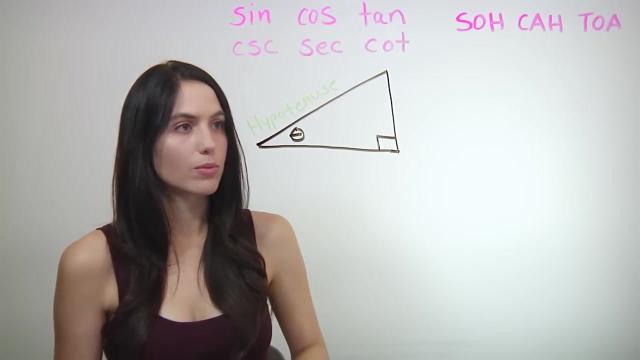 It's an angle that is not your right angle. What's important to know is what each of the sides of the triangle are in relation to theta. What I mean by that is, the longest side on the triangle is called the hypotenuse, So you'll just want to remember that the longest side is the hypotenuse. 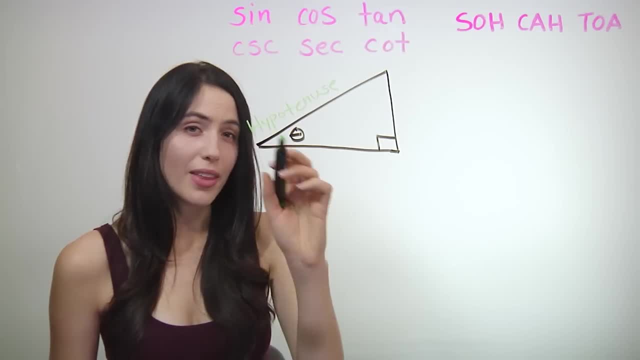 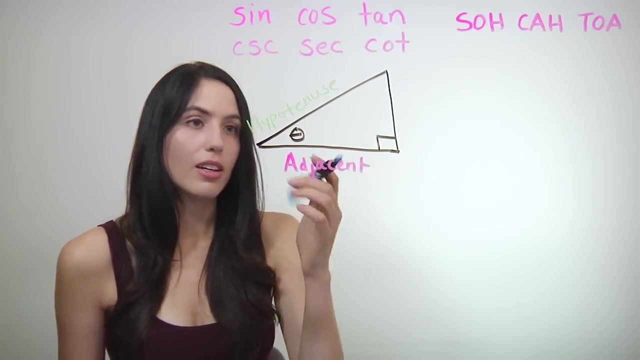 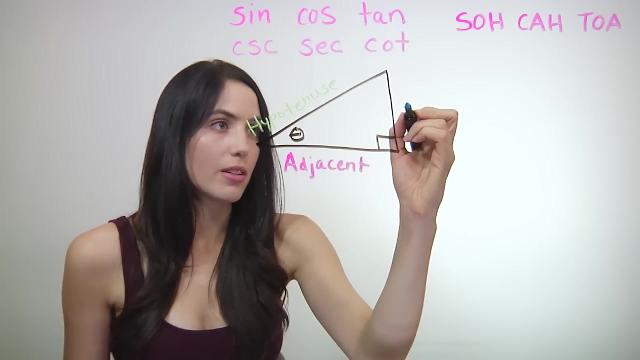 The other side that is next to theta, that is not the hypotenuse, is called the adjacent side. It's adjacent to theta, but it's not the hypotenuse. And the other side, the third side, is opposite theta, directly opposite theta, and it's the opposite side. 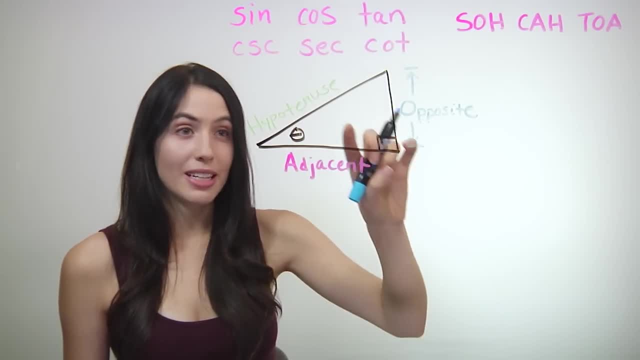 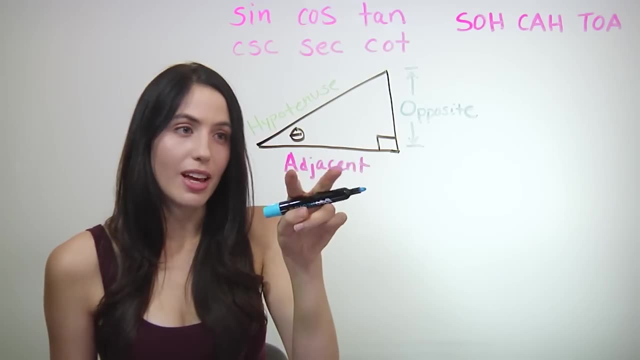 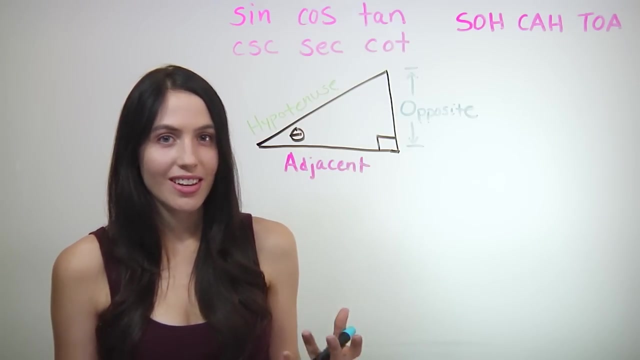 So notice that the hypotenuse is immediately opposite the right angle, the opposite side is opposite theta and then the adjacent side is the other side next to theta, that is not the hypotenuse. So you will use those to evaluate sine cosine and tangent. 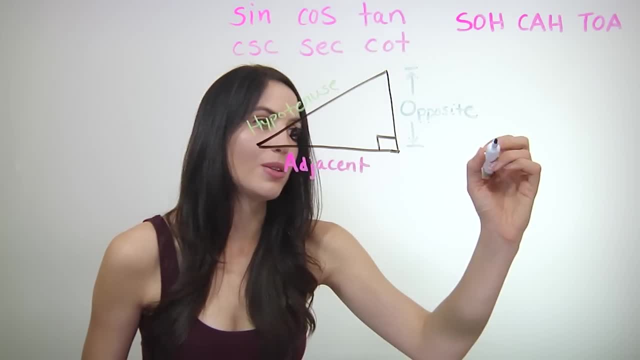 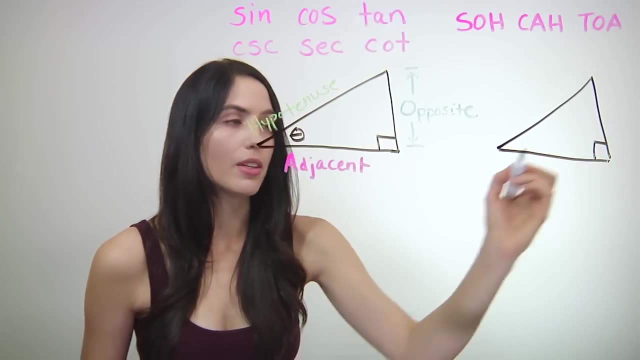 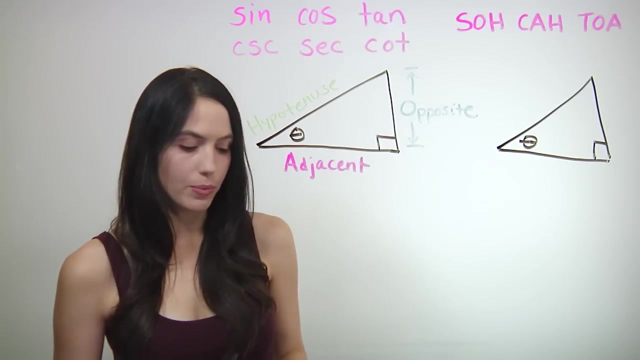 So you might be working on a problem that looks something like this where you're given triangle, you write triangle, the right angle, some theta labeled on your diagram and then side lengths that are given to you. So, for instance, you might be given that the longest side, the diagonal, is going to be 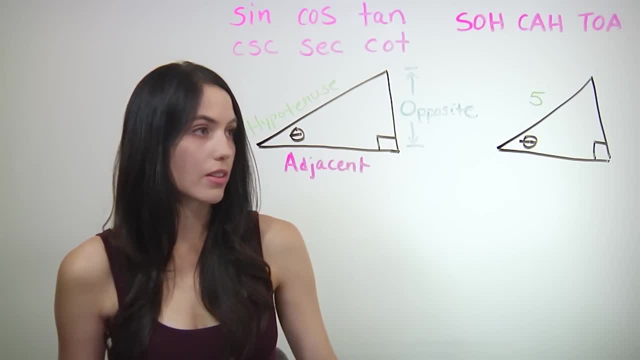 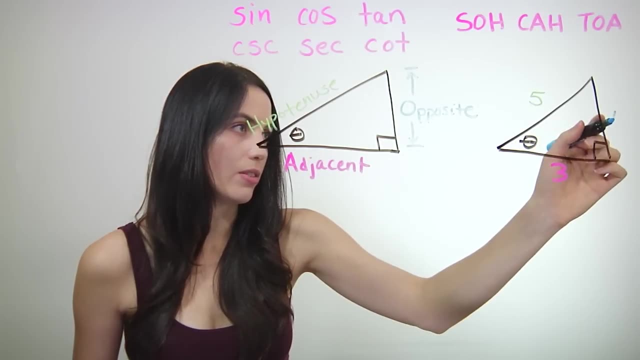 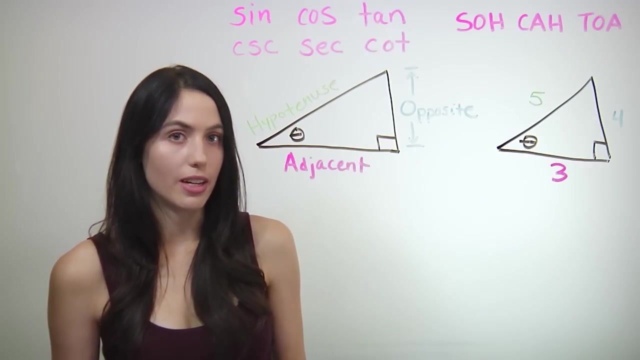 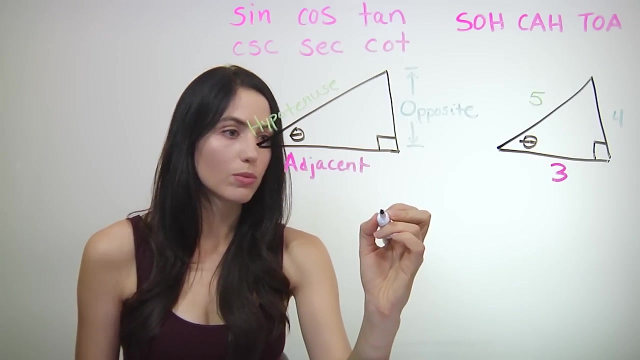 5,, this side length could be 3, and this side 4, and then the question might be: find sine of theta, cosine of theta and tangent of theta. So let's find those Sine of theta, Sine of theta. 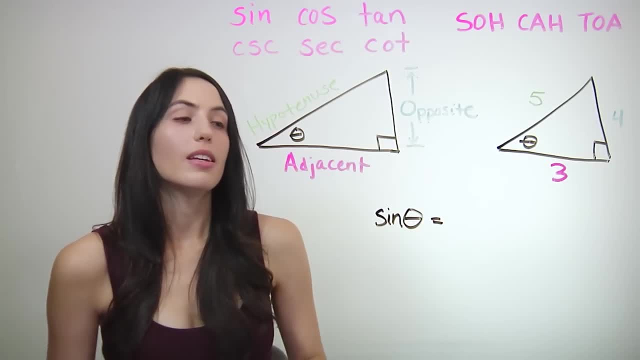 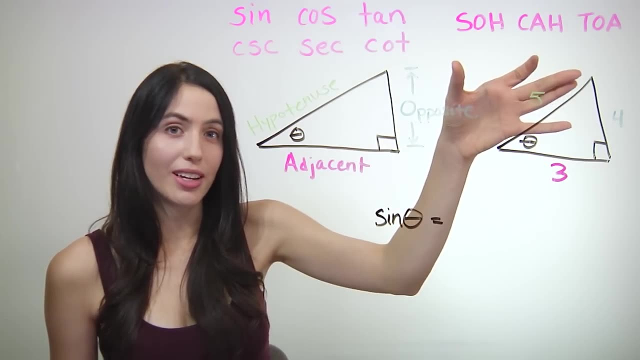 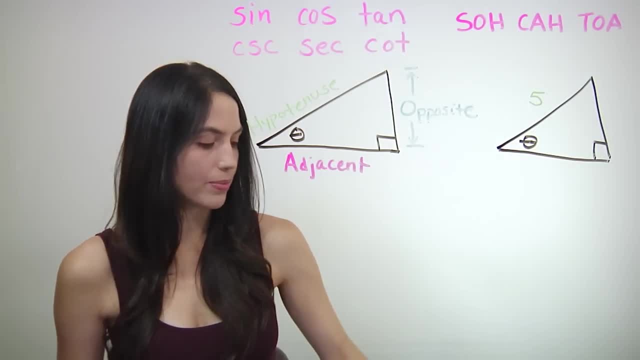 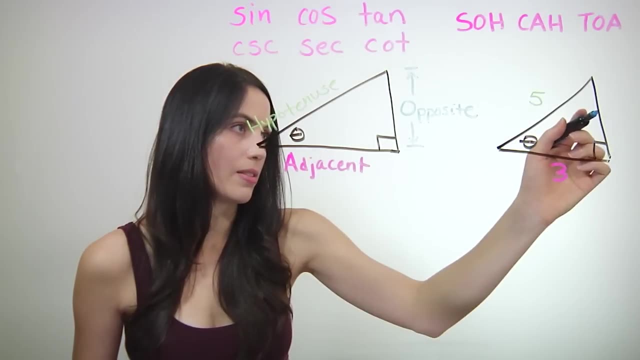 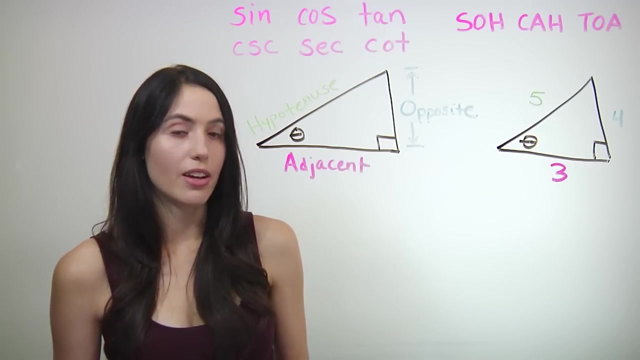 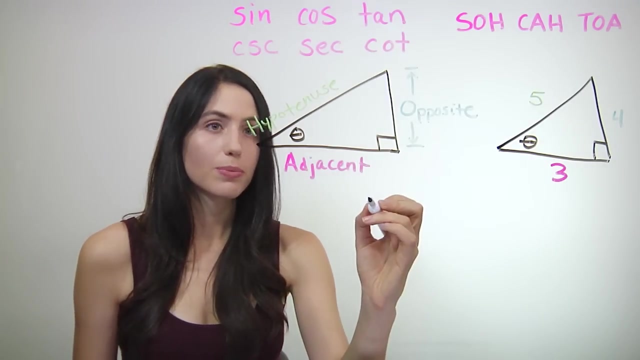 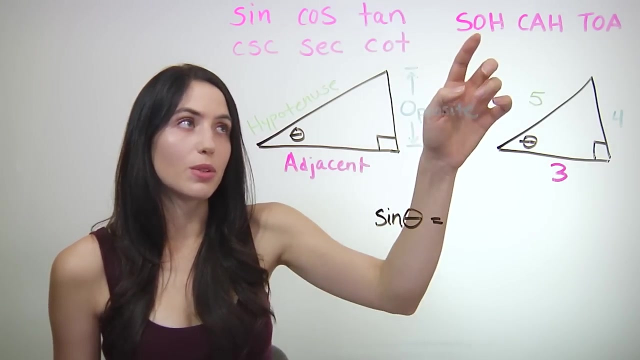 side of the diagonal is 5.. This side length could be 3, and this side 4.. And then the question might be: find sine of theta, cosine of theta and tangent of theta. So let's find those Sine of theta. sine of theta is equal to opposite over hypotenuse. 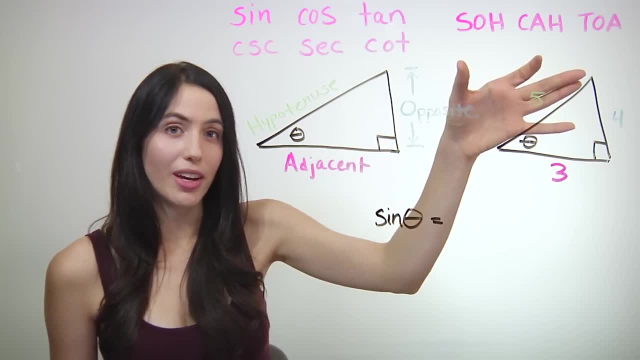 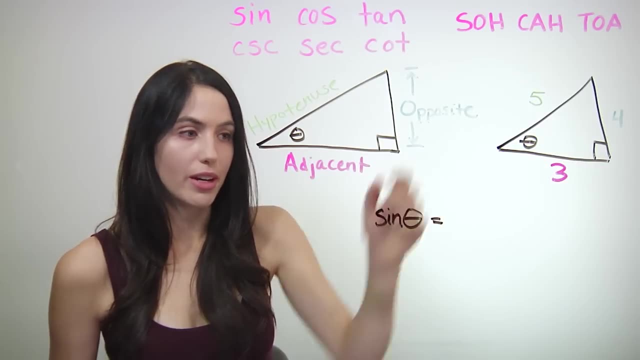 So this memory trick, SOHCAHTOA, can help you know what values to use for sine, cosine and tangent. For sine it's going to be opposite over hypotenuse. It's the SOH part of the memory trick. 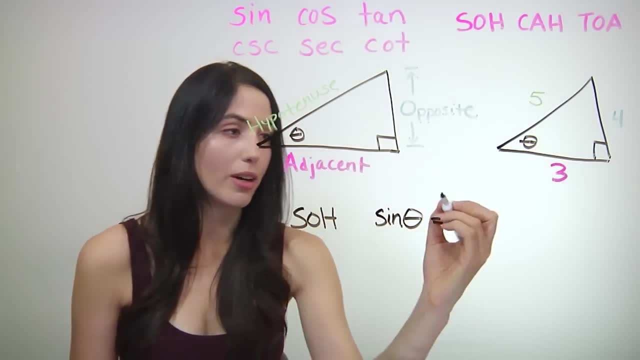 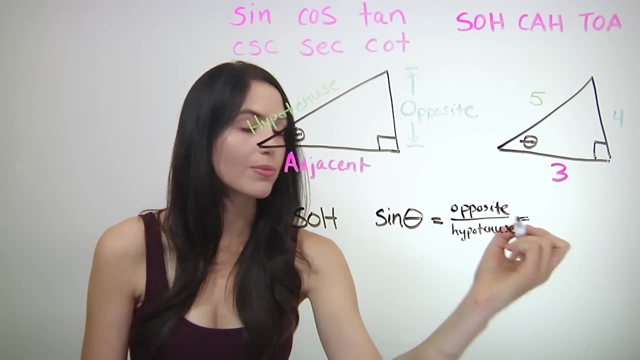 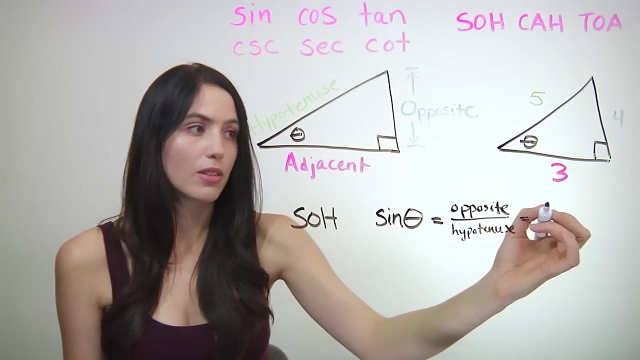 So sine equals, opposite over hypotenuse. So I'll write that out: Opposite over hypotenuse. And in this particular problem the opposite side is 4.. 4,, which is directly opposite theta, so you put 4, and the hypotenuse the longest side. 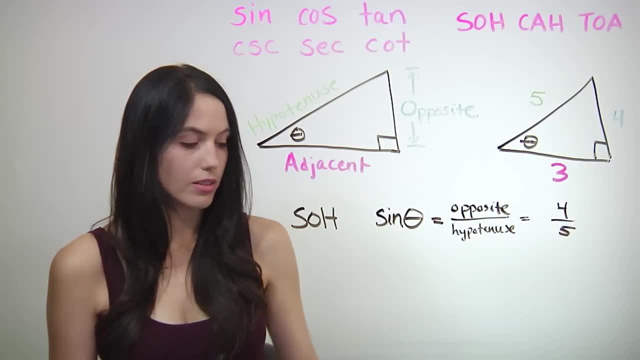 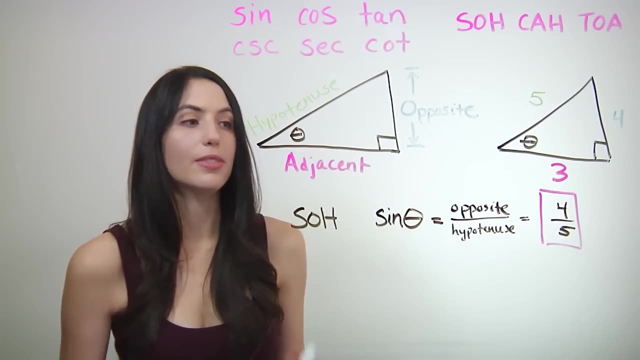 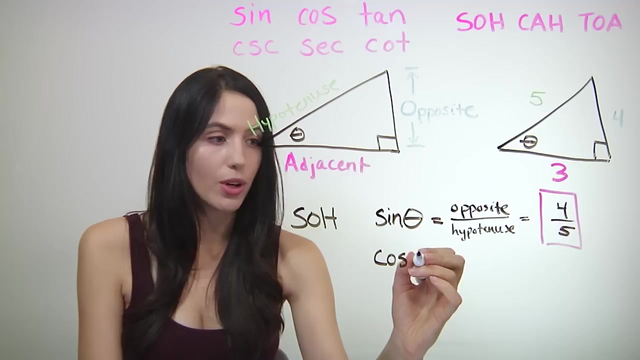 is 5, so you put 5.. So your answer for sine of theta is 4 fifths. In the same way, you can find cosine using your memory trick, the acronym SOHCAHTOA. So cosine is the C-A-H. 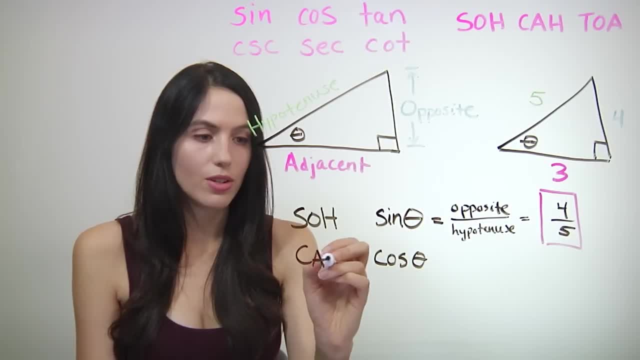 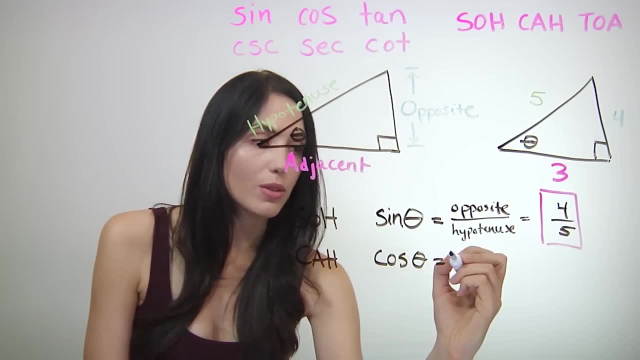 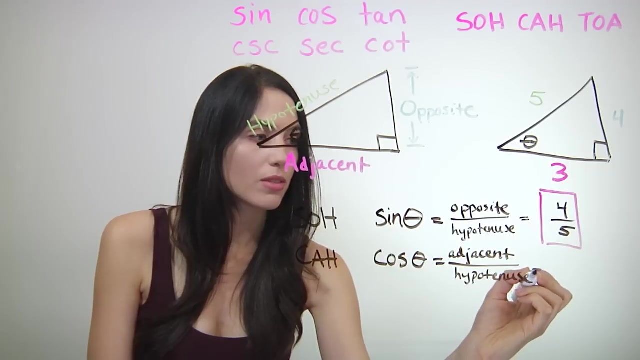 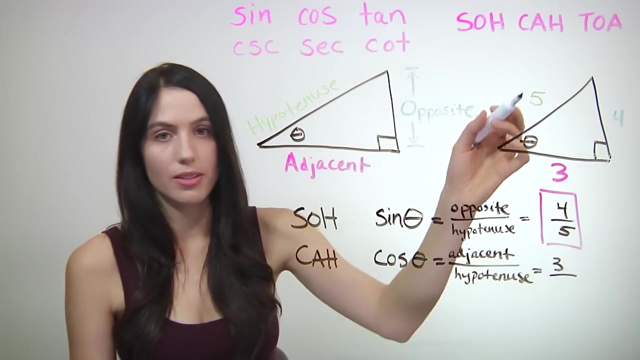 part of this trick, C-A-H, and that stands for cosine equals adjacent over hypotenuse- Cosine equals adjacent over hypotenuse, and so in this problem the adjacent side to theta is 3, and the hypotenuse is again 5. So your cosine value is 3 fifths. 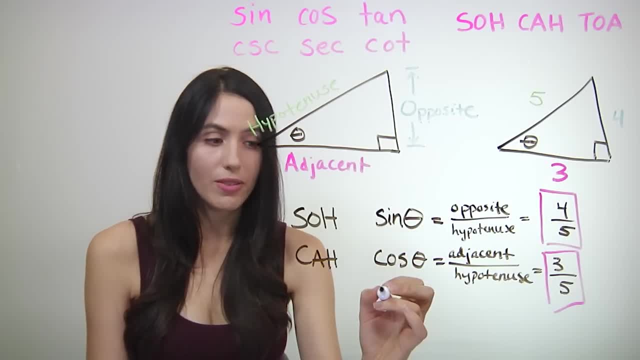 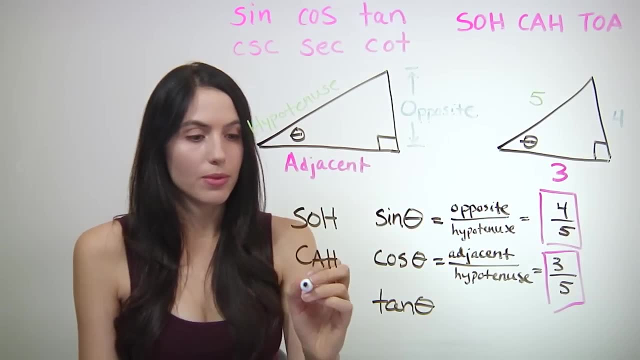 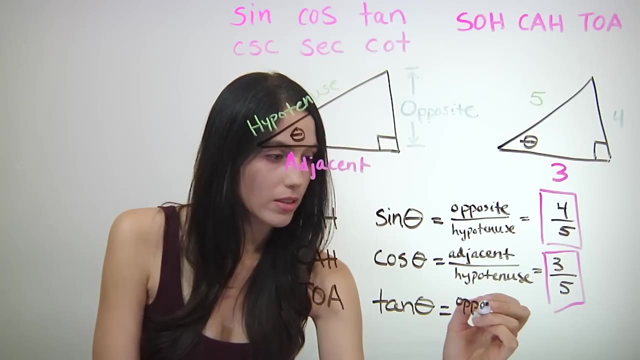 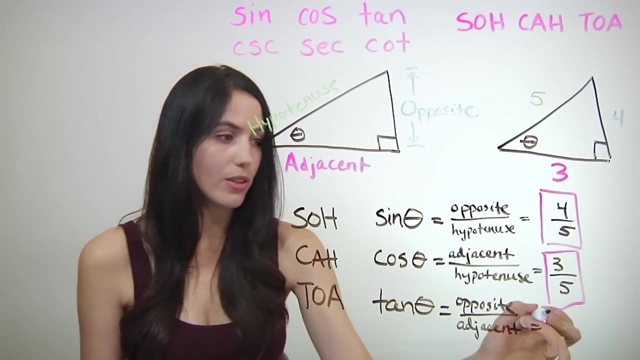 And then, finally, if you have to find tangent of theta, just remember this part of the name: SOHCAHTOA, the TOA part T-O-A. so tangent equals opposite over adjacent. The opposite side in this triangle is 4, and the adjacent side is 3,, so you have 4 over 3.. So your tangent. 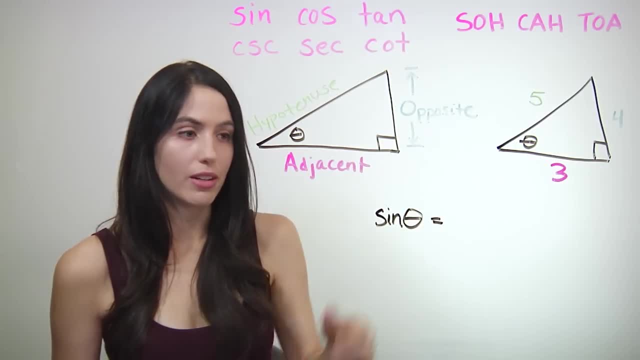 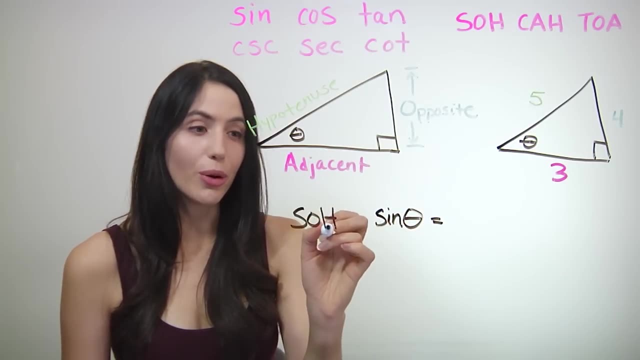 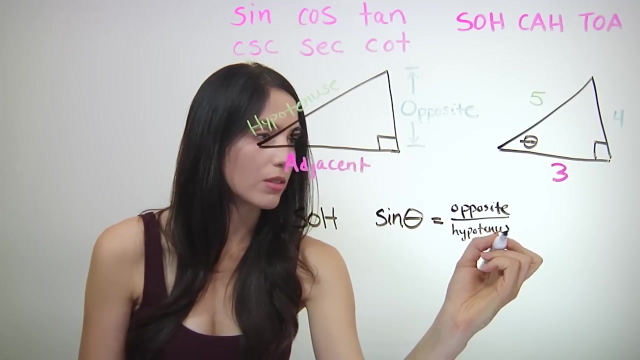 and tangent For sine. it's going to be opposite over hypotenuse. It's the SOH part of the memory trick. So sine equals opposite over hypotenuse. So I'll write that out: opposite over hypotenuse. and in this particular problem you're going. 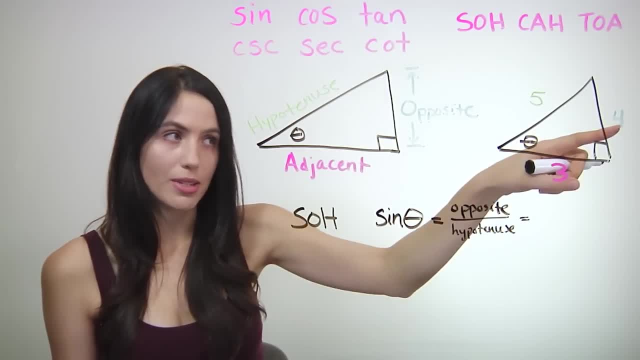 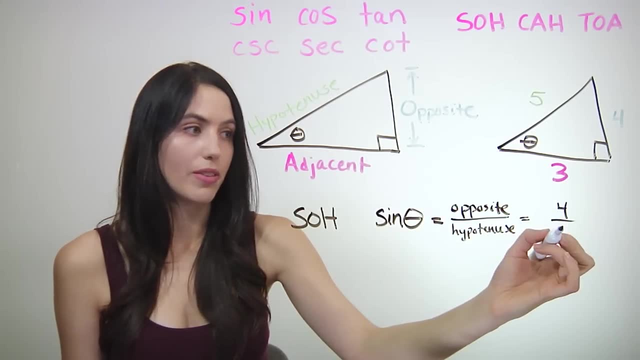 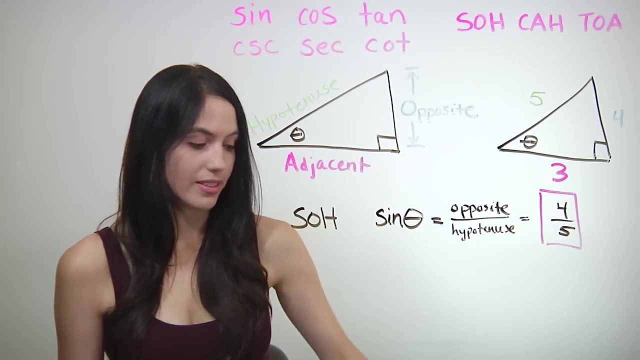 to have. the opposite side is 4,, which is directly opposite theta, so you put 4, and the hypotenuse the longest side is 5,, so you put 5.. So your answer for sine of theta is 4. fifths, 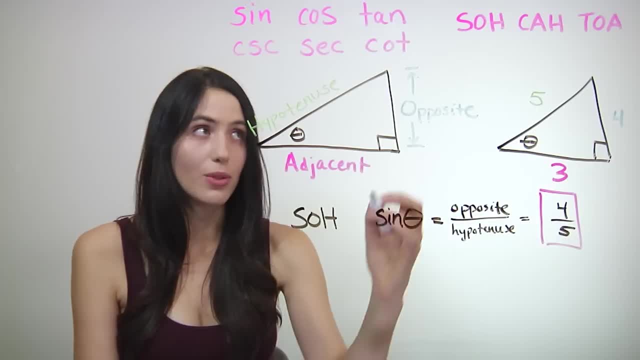 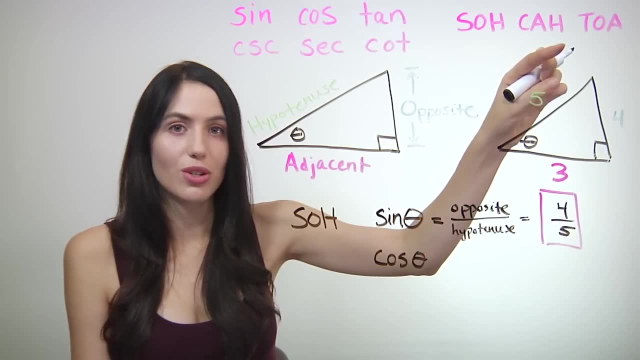 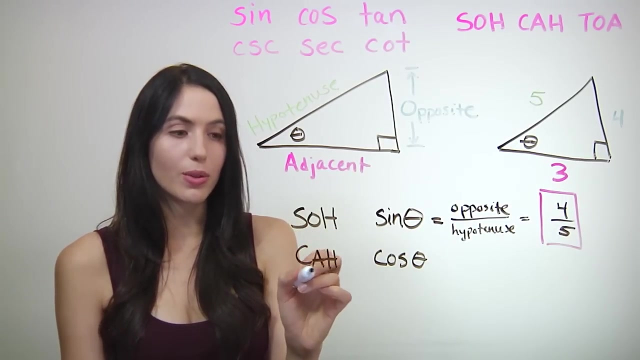 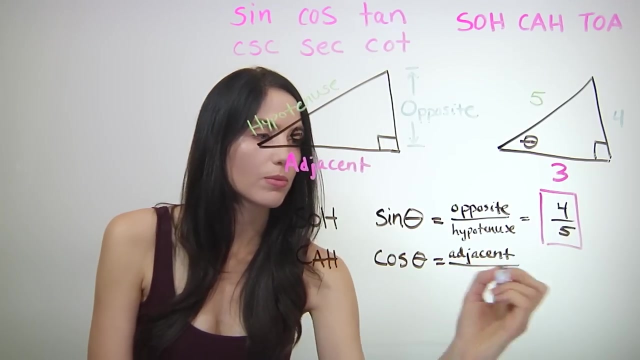 In the same way you can find cosine using your memory trick, the acronym SOH, CAH, TOA. So cosine is the CAH part of the memory trick. CAH and that stands for cosine, equals adjacent over hypotenuse, and so in this problem the 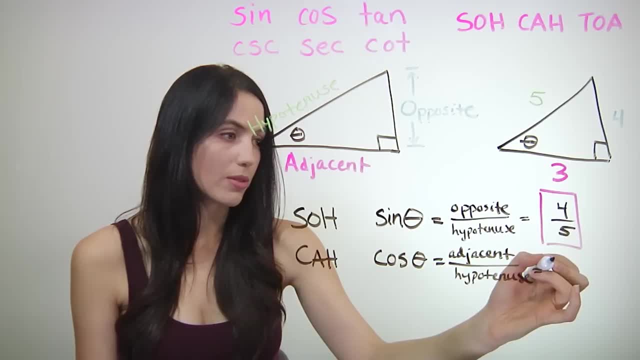 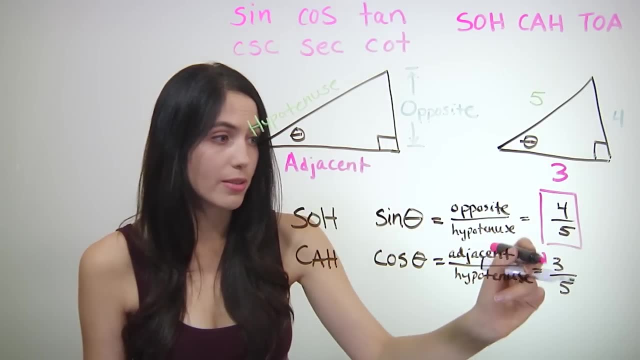 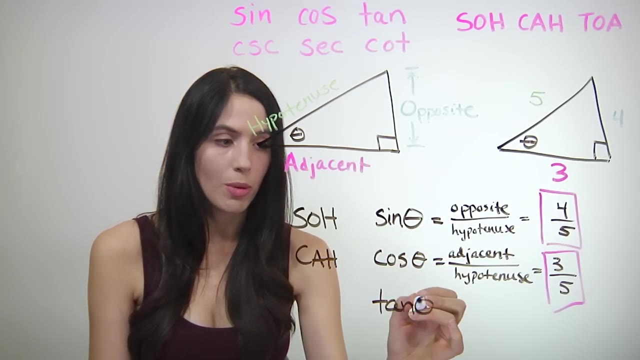 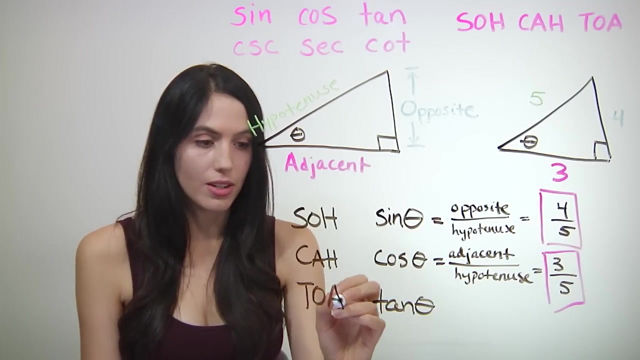 adjacent side to theta is 3, and the hypotenuse is again 5,, so your cosine value is 3 fifths. And then finally, if you have to find tangent of theta, just remember this part of the name: SOH, CAH, TOA, the TOA part T-O-A. so tangent equals opposite over adjacent. 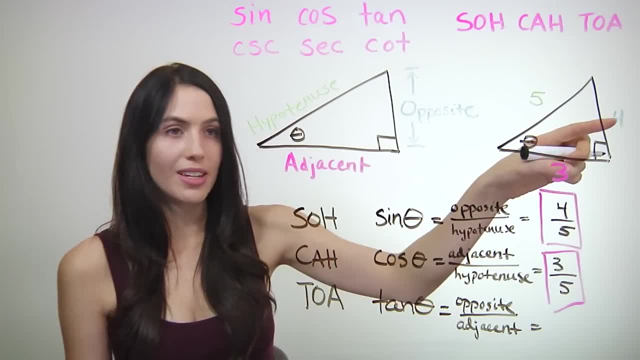 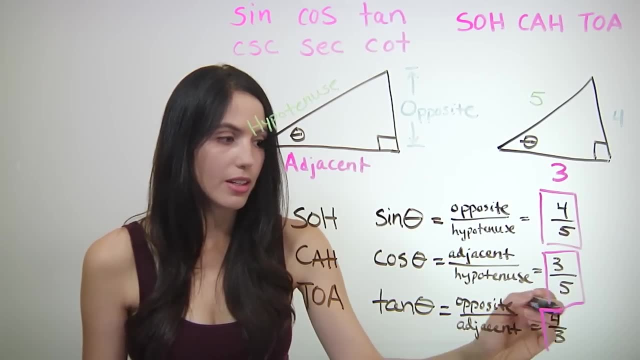 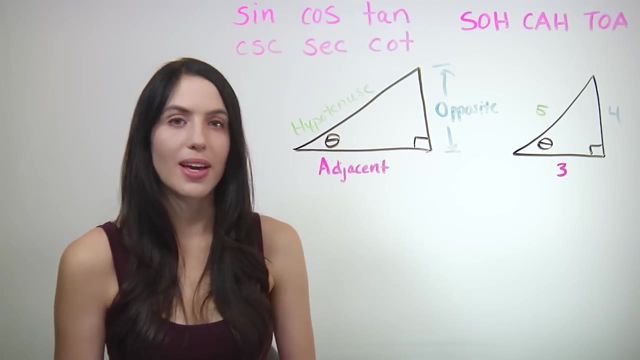 The opposite side in this triangle is 4, and the adjacent side is 3,, so you have 4 over 3.. So your tangent of theta equals tangent over theta. So your tangent of theta equals 4 thirds. Okay, say you actually need to find the values of cosecant, secant or cotangent, one of. 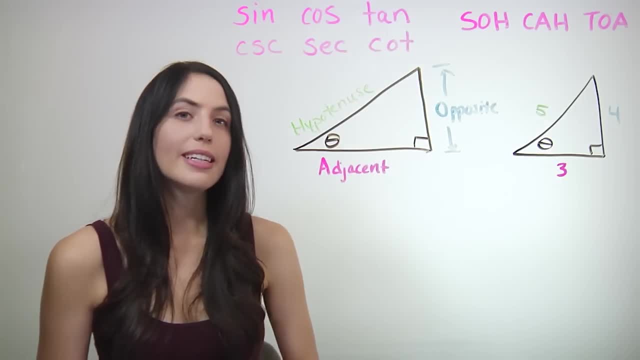 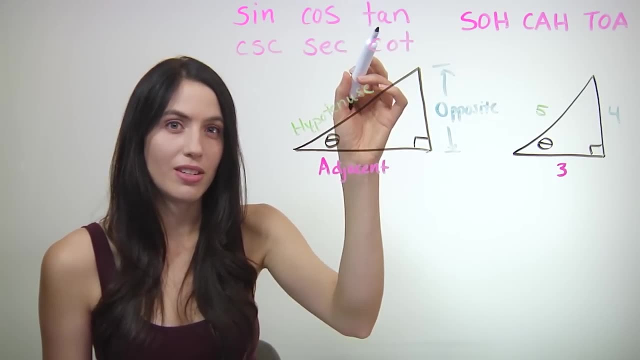 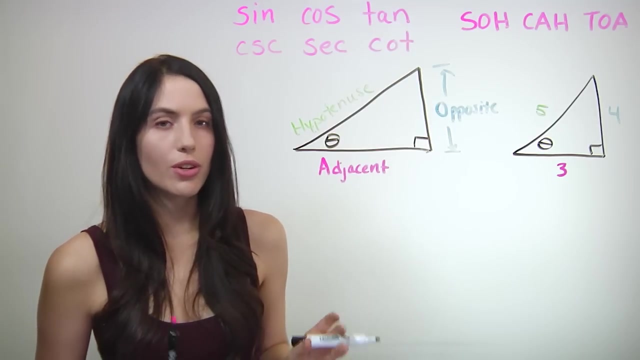 the other three basic trig functions. The easiest way is to first find the value of their partner trig functions- sine, cosine or tangent- and then take the reciprocal 1 over sine, 1 over cosine, 1 over tangent. So let me show you how to do that. 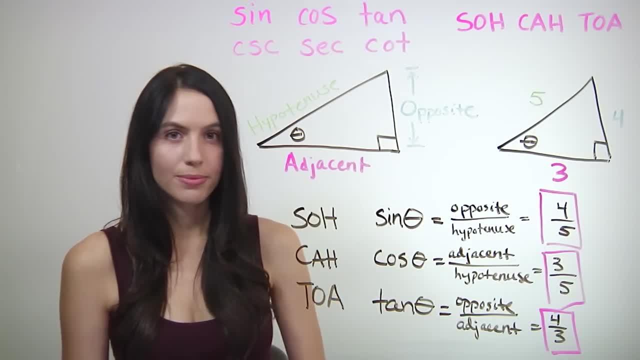 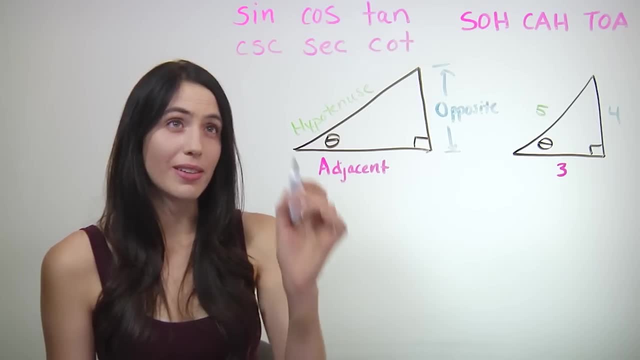 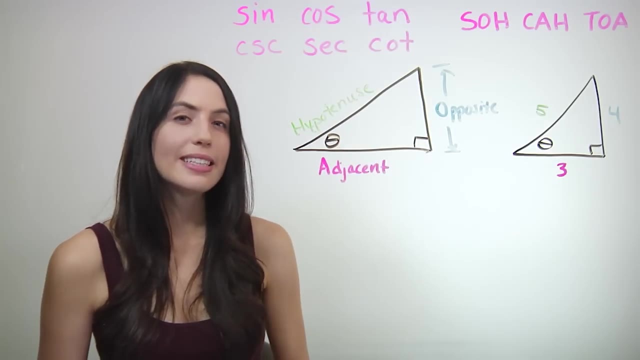 of theta. So you're going to find the value of tangent of theta equals 4 thirds. OK, Say you actually need to find the values of cosecant, secant or cotangent, one of the other three basic trig functions. The easiest way is to first find the value of. 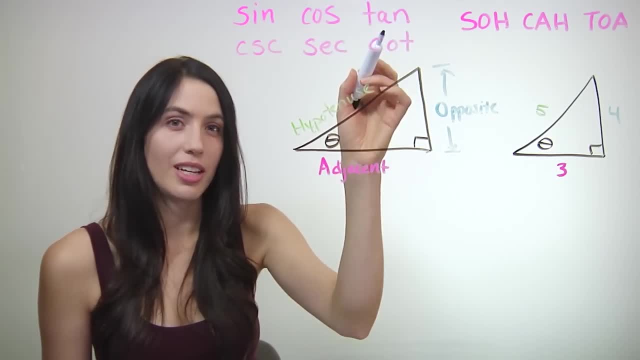 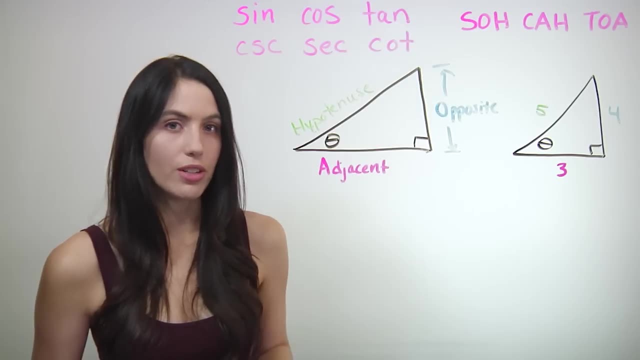 their partner trig functions sine cosine or tangent, and then take the reciprocal 1 over sine, 1 over cosine, 1 over tangent. So let me show you an example. Say you wanted to find cosecant of theta. 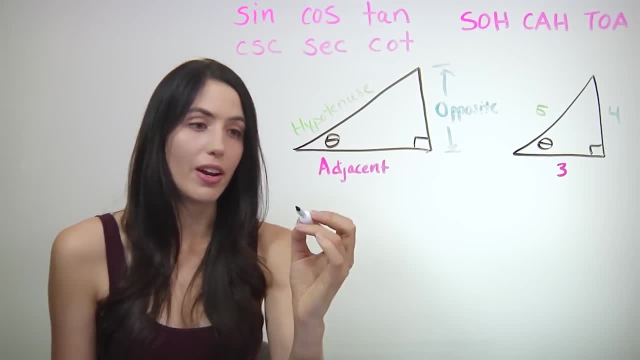 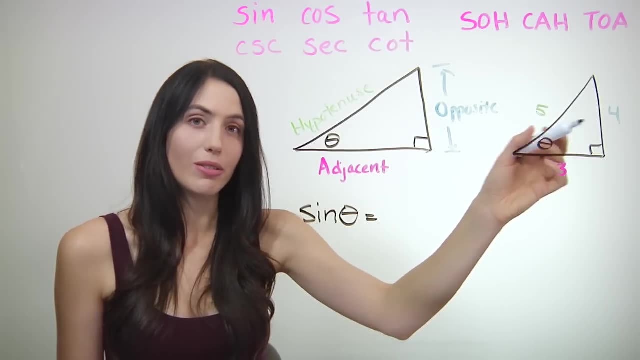 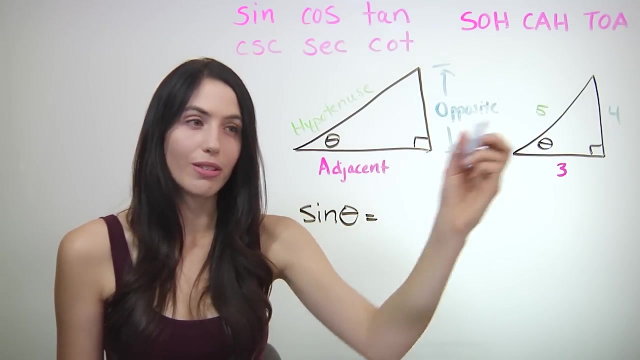 csc of theta. First find its partner sine of theta. And in this example, sine of theta, remember, is opposite over hypotenuse from SOHCAHTOA. Sine is opposite over hypotenuse. So in this triangle it is 4 over 5.. 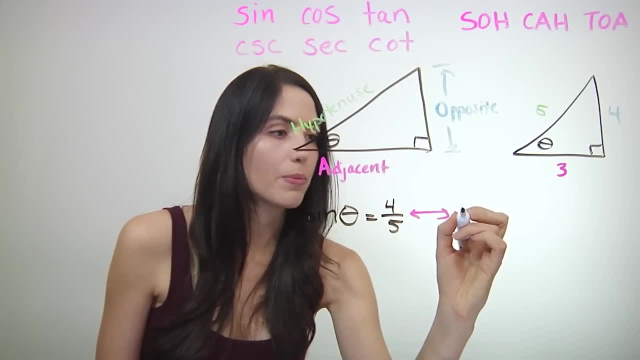 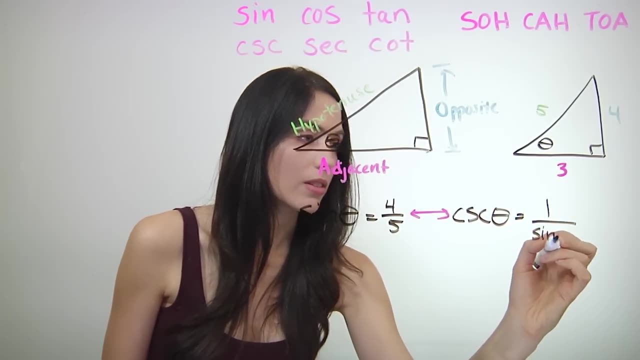 COSECANT, COSECANT, COSECANT, COSECANT, COSECANT, COSECANT, COSECANT of theta is, by definition, 1 over sine theta, And what that really means is that you can just flip numerator and denominator of sine. 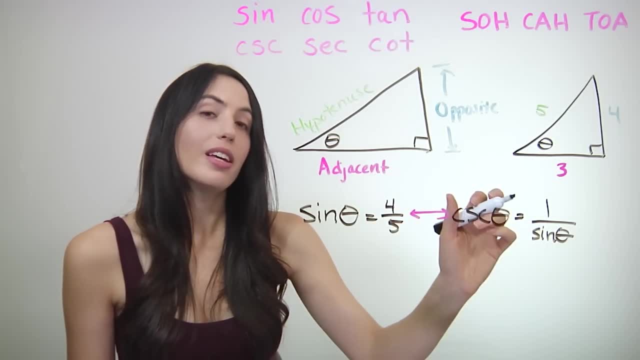 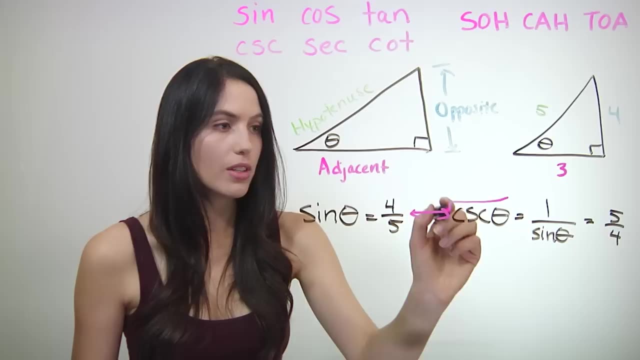 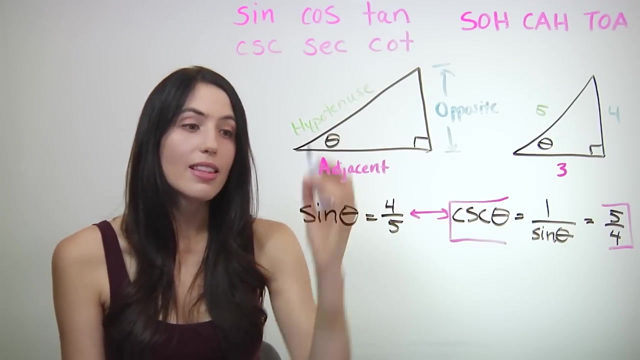 flip top and bottom. So instead of 4 over 5, it's 5 over 4 for cosecant theta. So your cosecant theta equals 5 fourths. Now if you wanted to find secant theta, sec theta, you would first find cosine theta. 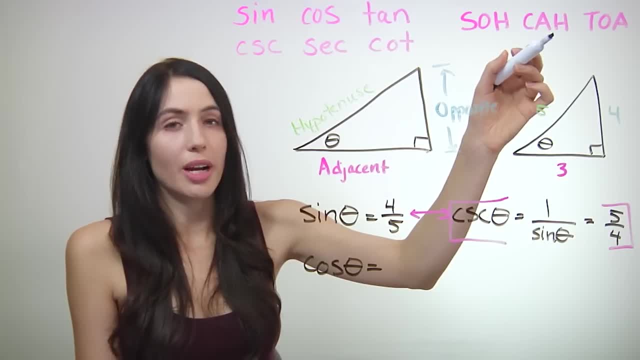 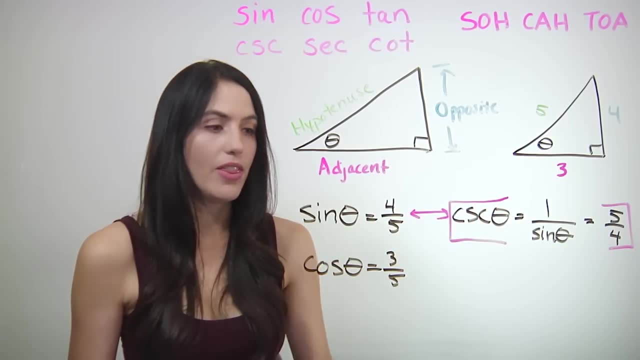 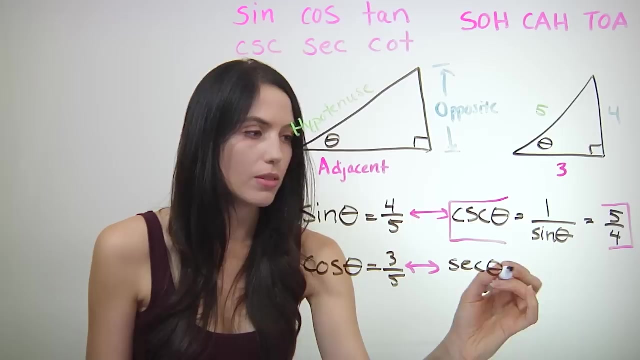 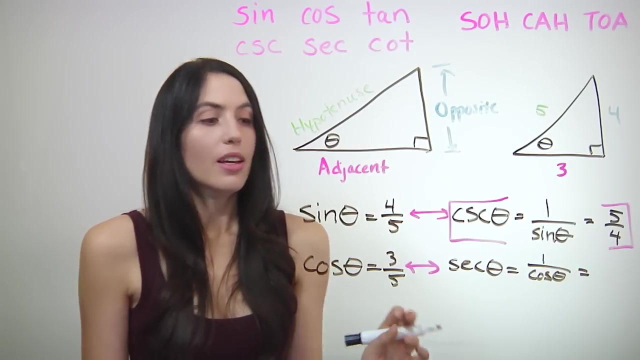 In this triangle, remember, cosine is adjacent over hypotenuse, so here it's 3 over 5.. Then to get secant theta, sec theta, you would take 1 over cosine theta, And that can be found just by flipping top and bottom. 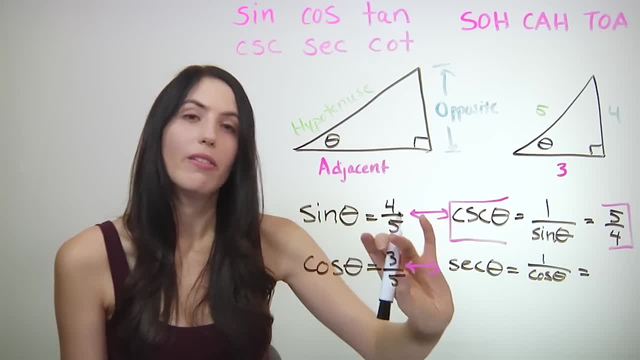 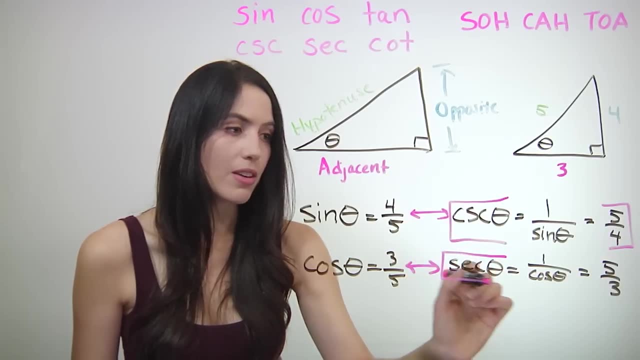 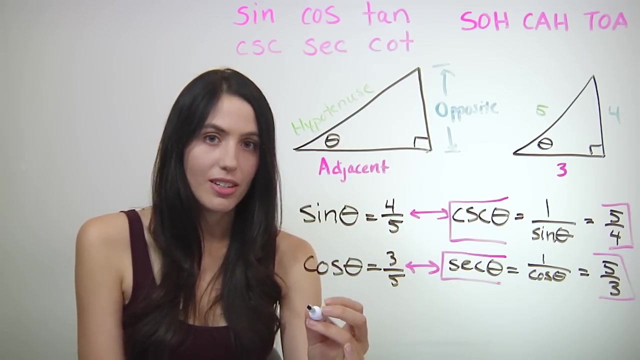 So instead of 3 over 5, 1 over that would turn out to be 5 over 3, the reciprocal So we have secant theta's value is 5 thirds. And then, finally, if you wanted to find cotangent theta, you would first find tangent theta. 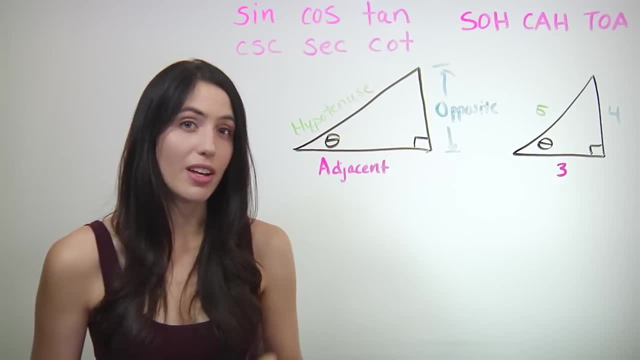 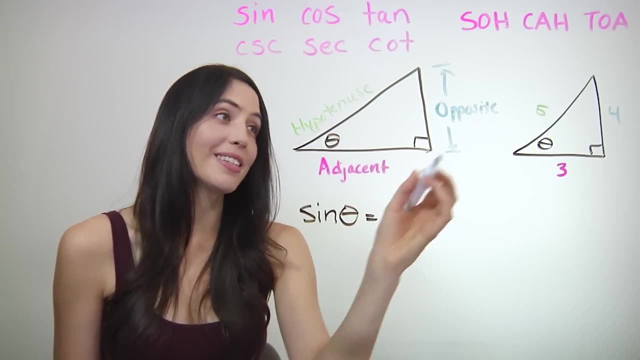 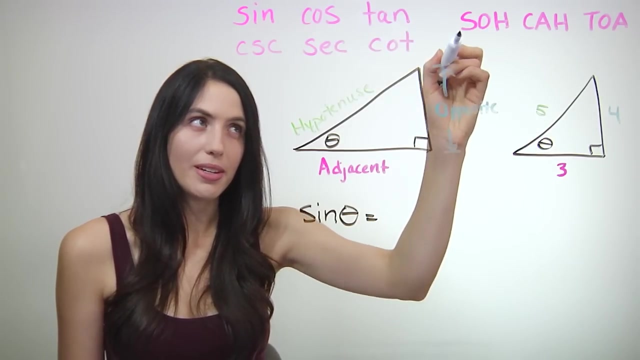 Let me give you an example. Say you wanted to find cosecant of theta, C-S-C, theta First, find its partner sine of theta. and in this example, sine of theta, remember, is opposite over hypotenuse from SOH CAH TOA. 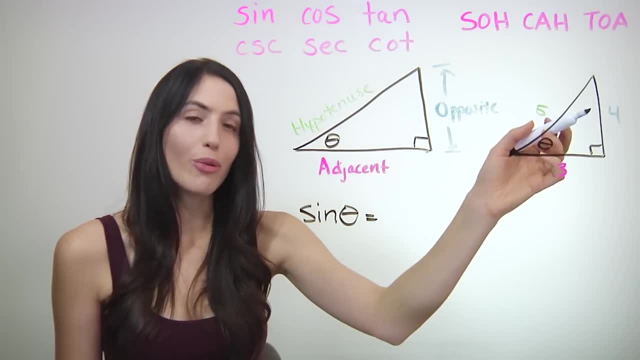 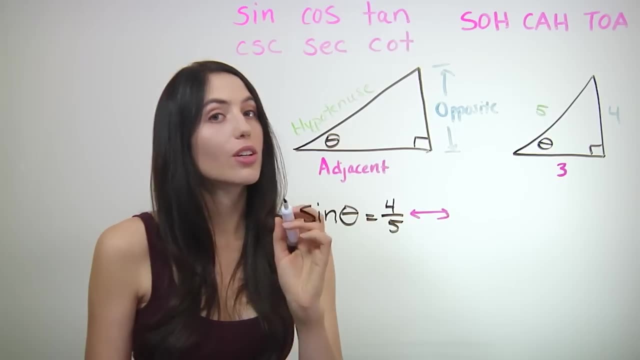 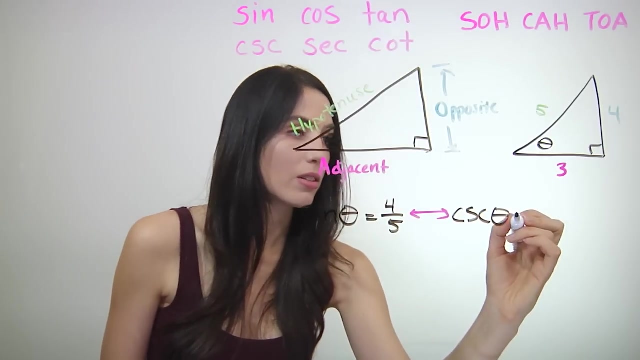 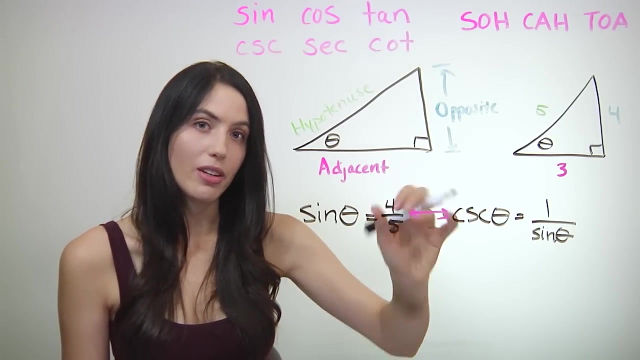 Sine is opposite over hypotenuse, so in this triangle it is 4 over 5.. Secant of theta is by definition 1 over sine theta, And what that really means is that you can just flip numerator and denominator of sine. 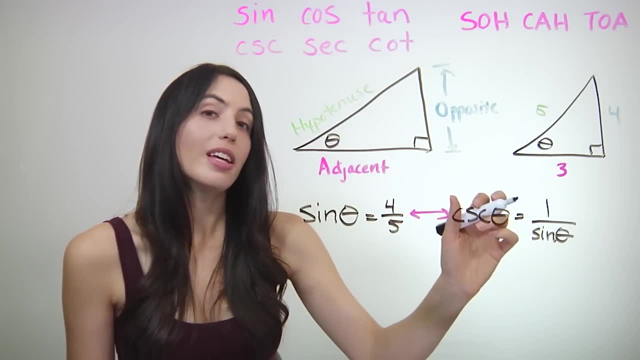 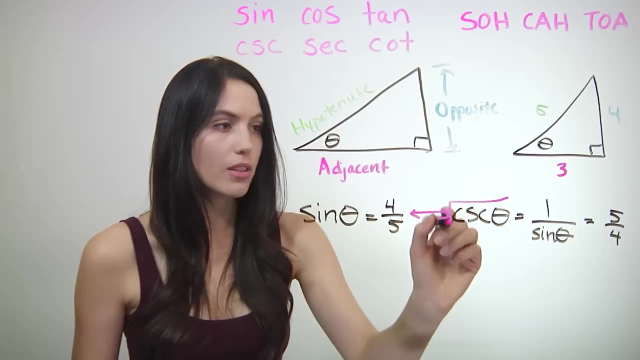 Flip top and bottom. So instead of 4 over 5, it's 5 over 4, or cosecant theta. So your cosecant theta equals 5 fourths. Now, if you wanted to find secant, you would just look at this first. on the table right: 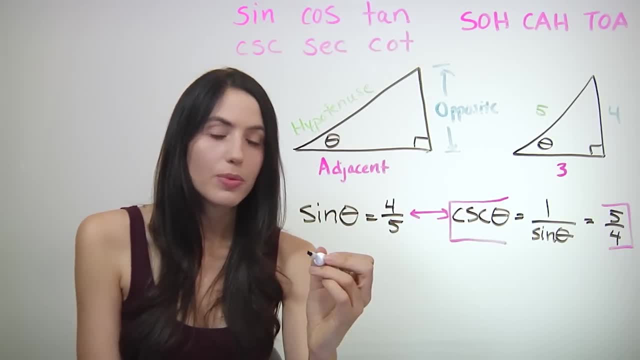 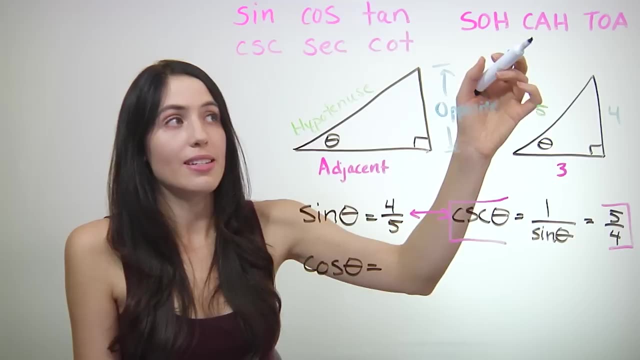 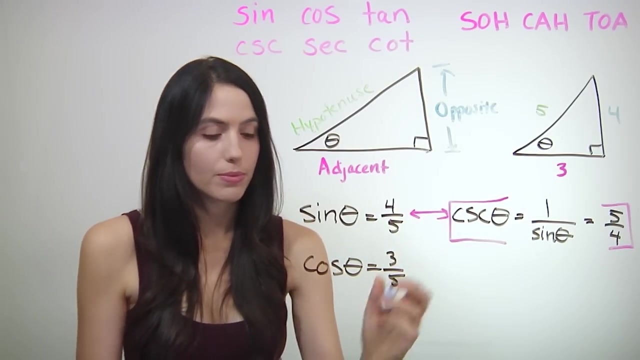 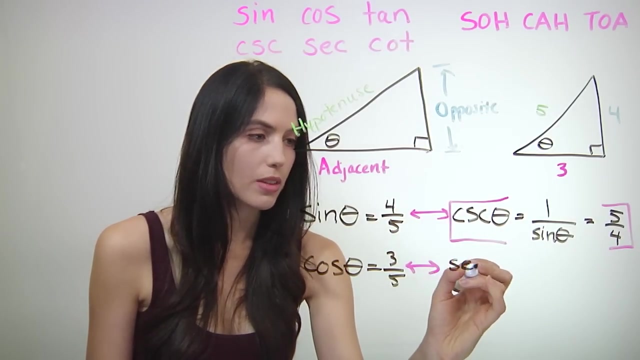 There's no second secant theta, sec theta. you would first find cosine theta In this triangle. remember, cosine is adjacent over hypotenuse, so here it's 3 over 5.. Then to get secant theta, sec theta. 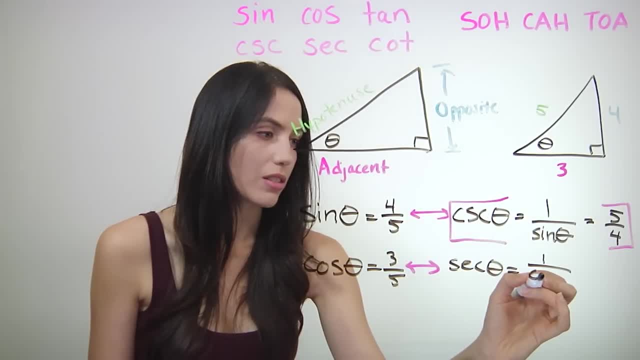 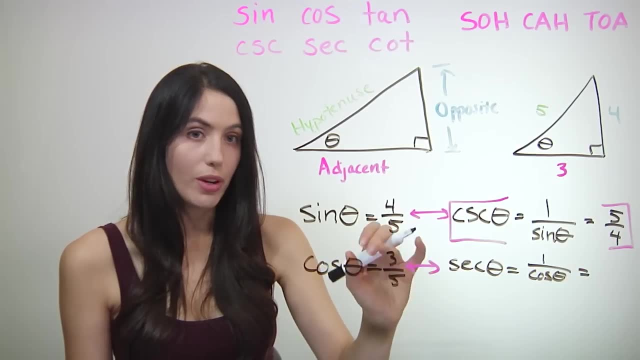 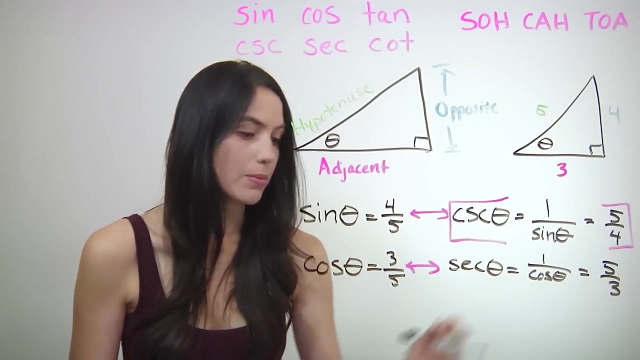 you would take 1 over cosine theta And that can be found just by flipping top and bottom. So instead of 3 over 5, 1 over that would turn out to be 5 over 3, the reciprocal So we have secant theta's value is 5 thirds. 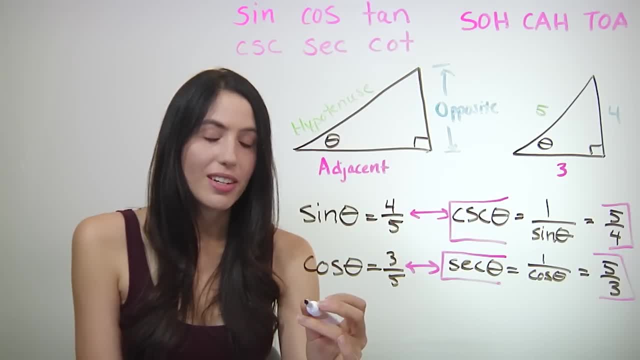 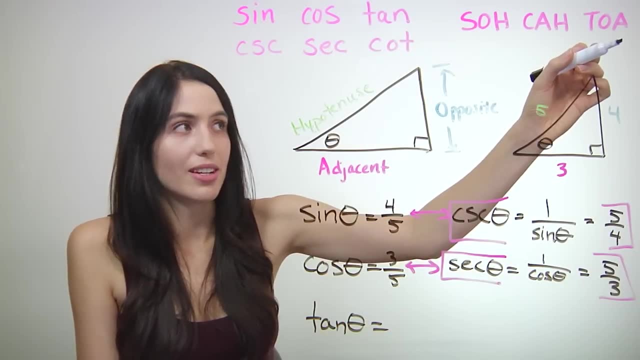 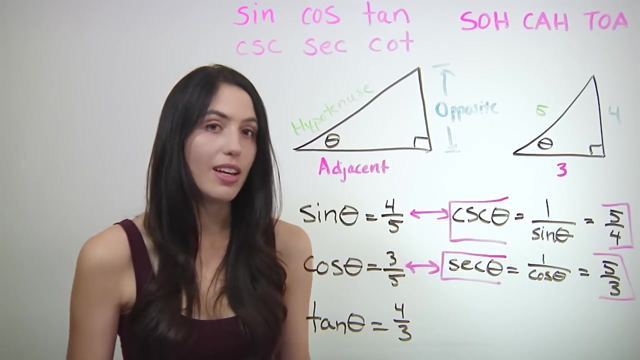 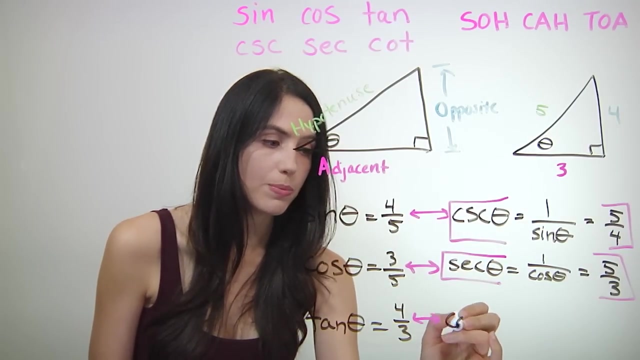 And then, finally, if you wanted to find cotangent theta, you would first find tangent theta. So tangent theta Is opposite over adjacent, So in this triangle it's 4 over 3.. And then to get cotangent, you would do 1 over tangent. 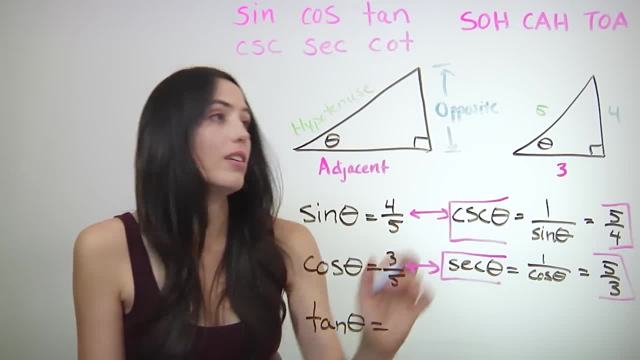 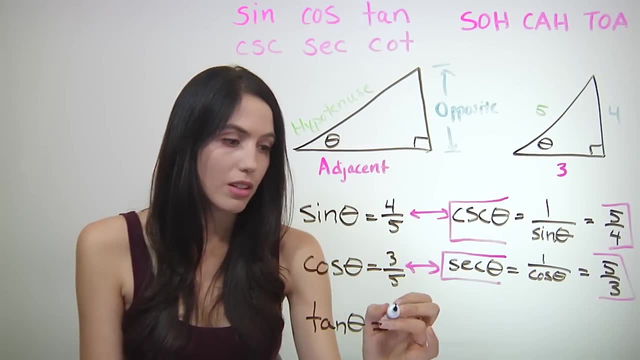 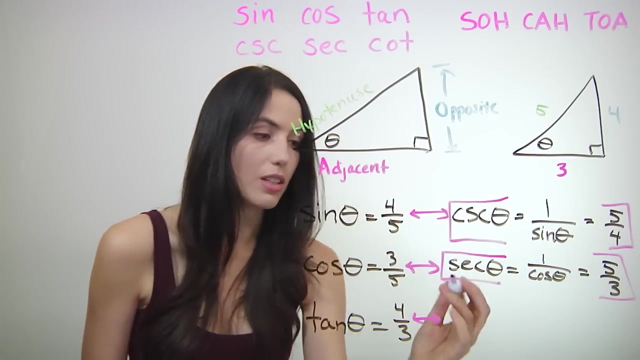 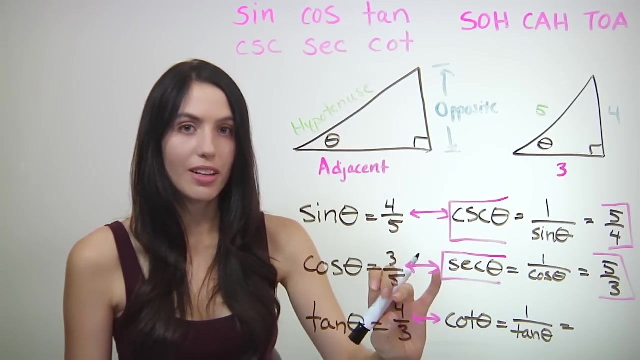 So tangent theta is 1 over cosine theta, So that's 1 over cosine theta. It's opposite over adjacent, So in this triangle it's 4 over 3.. And then to get cotangent, you would do 1 over tangent, which is the reciprocal of this. 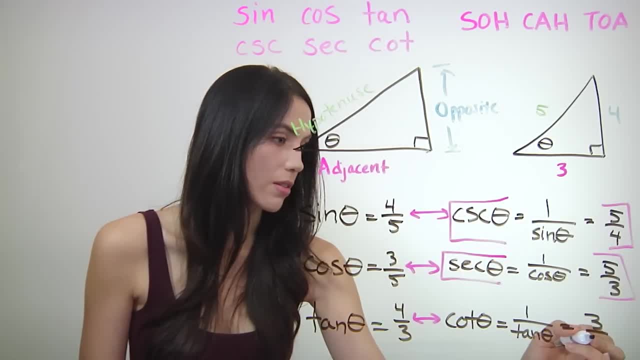 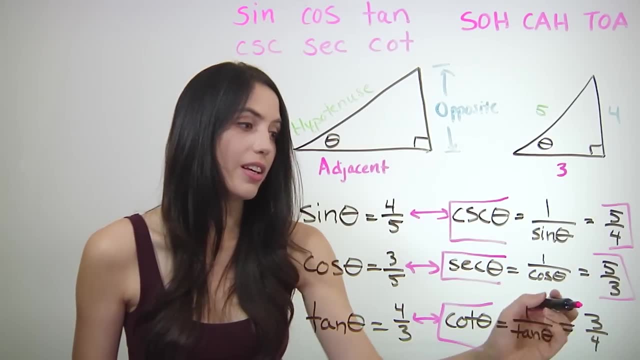 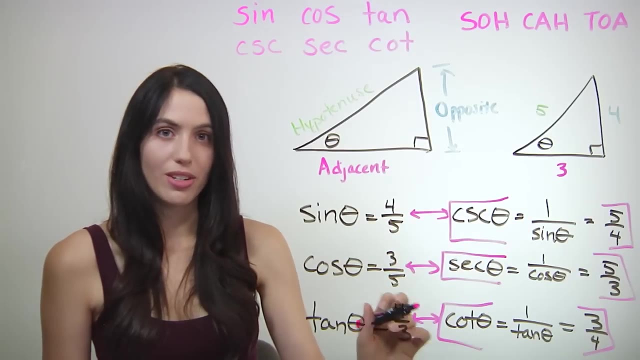 value. So it's 3 over 4.. Cotangent of theta is 3 fourths. That is the fastest, easiest way to find cosecant, secant and cotangent. Okay, I want to show you some things that can trip people up. 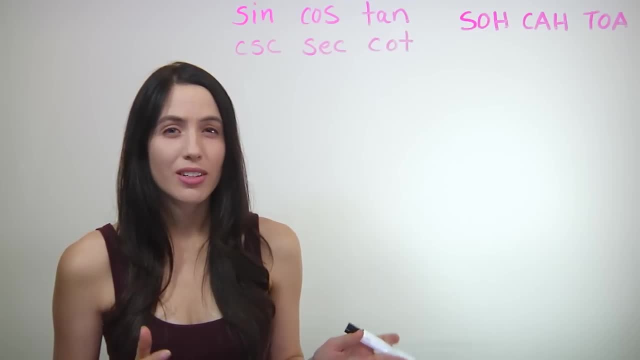 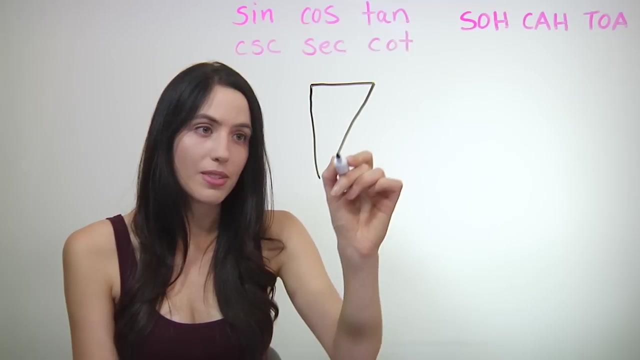 One thing that confuses people is when the right triangle is drawn at a different orientation, So if it's sideways or on its hypotenuse. So, for instance, You could have a triangle that's drawn like this, It's still a right triangle. 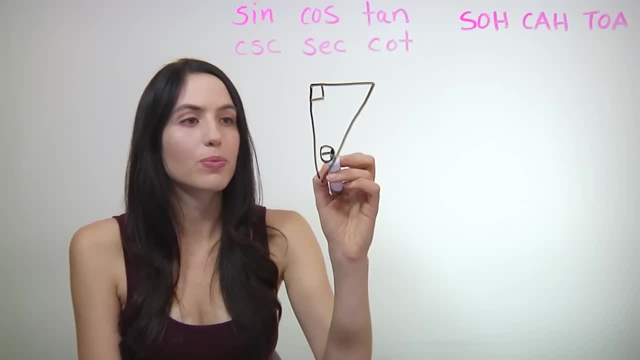 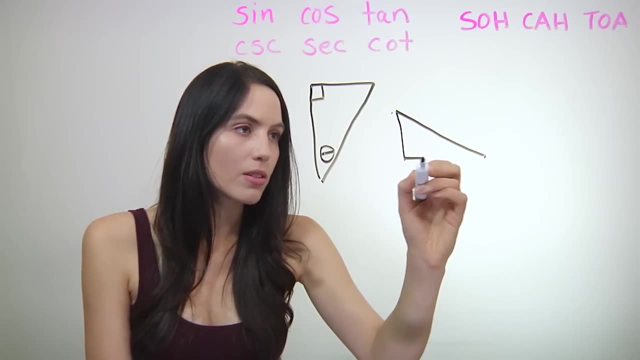 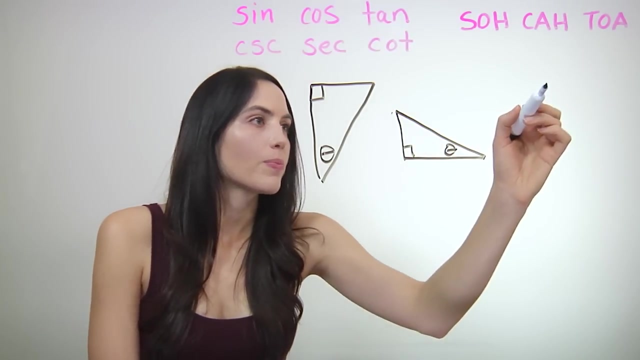 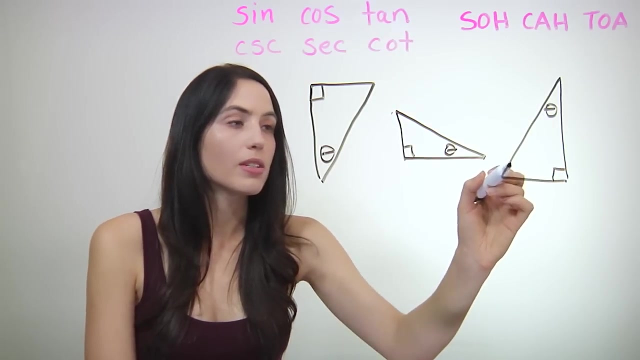 It looks kind of upside down. Your theta could be here. You could have a triangle that looks like this. So it's the reverse of the one in our example. You could have a triangle drawn with your theta- Okay, With your theta up here instead of down here. 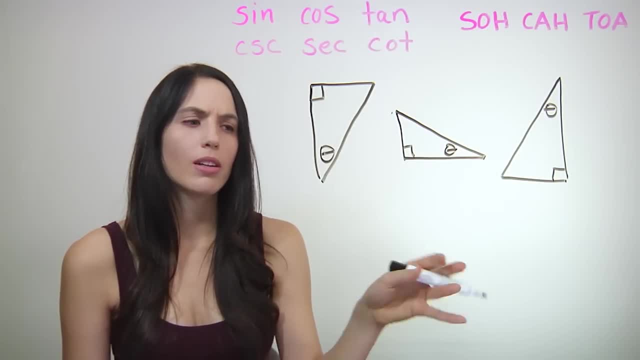 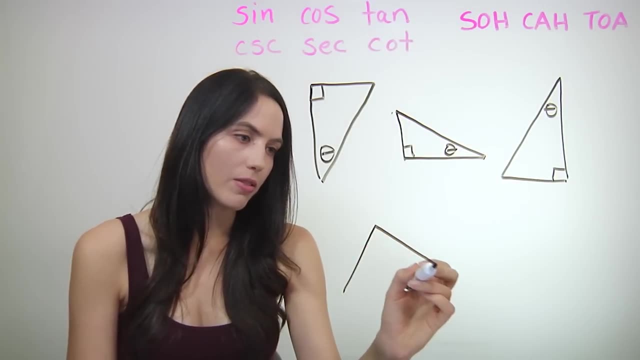 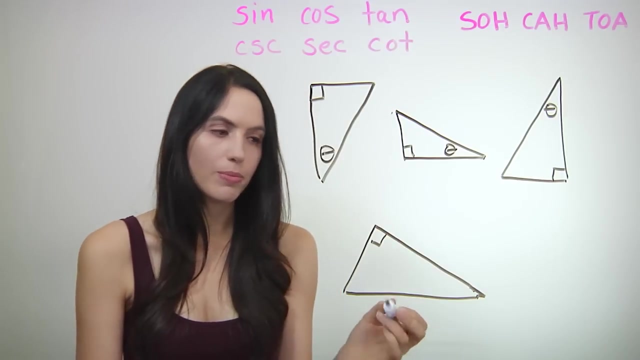 And the one that's most confusing to people is when the right triangle is drawn so that its hypotenuse is horizontal. It's sort of on the ground. So here's an example of that: If your right angle was actually up here, then your hypotenuse turned out to be horizontal. 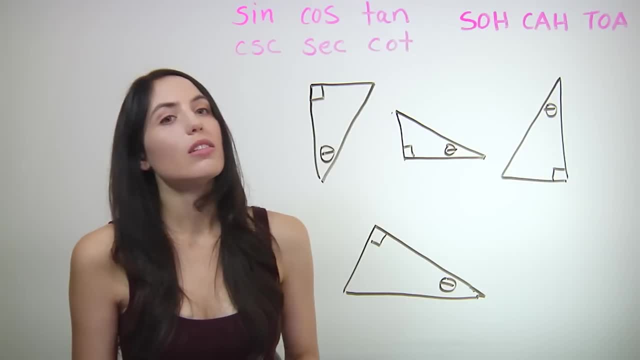 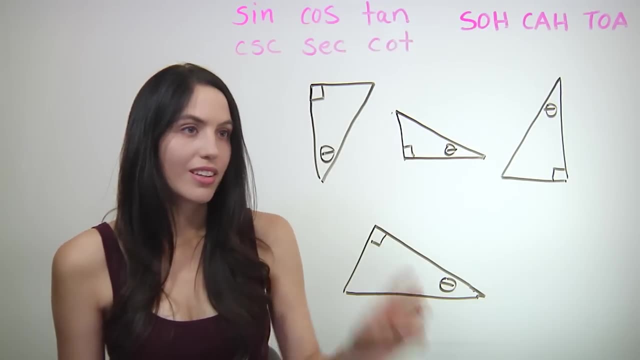 And your theta could be here or here. So let's look at these examples And label where your opposite, adjacent and hypotenuse are. for these triangles In this example and all of these triangles actually, you can rely on your hypotenuse being the longest side. 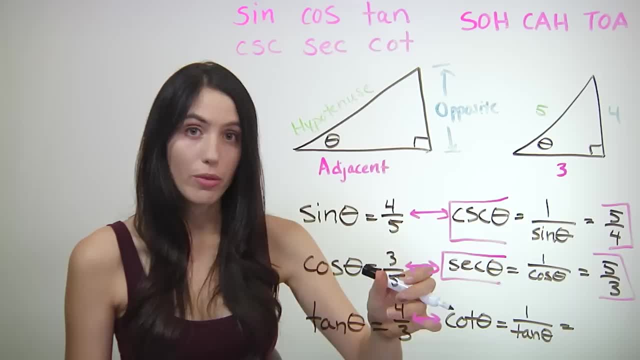 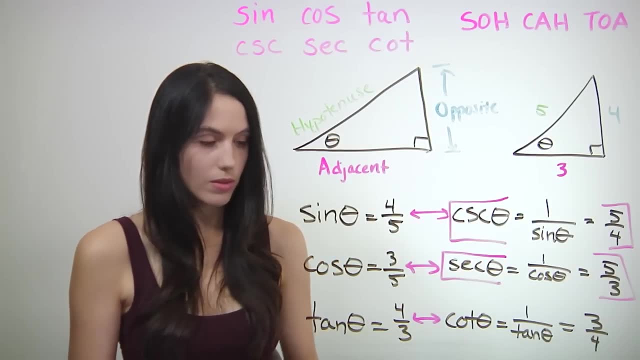 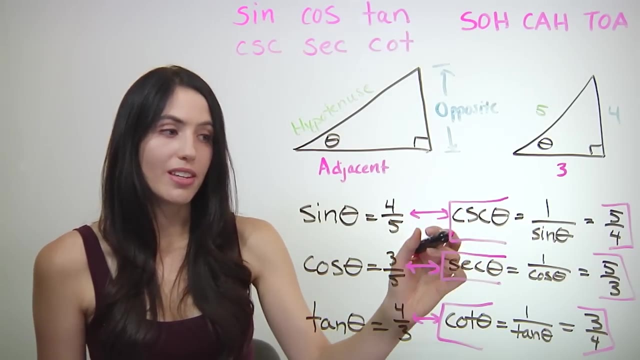 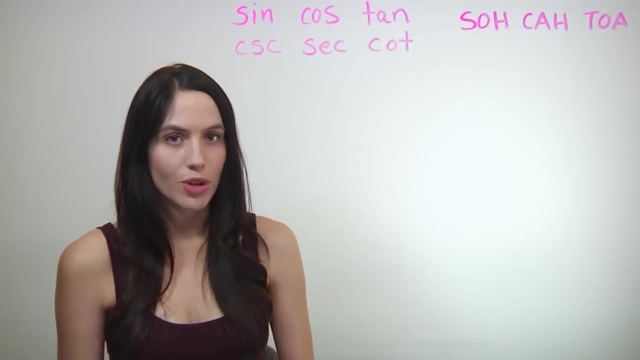 which is the reciprocal of this value. so it's 3 over 4.. Cotangent of theta is 3 fourths. That is the fastest, easiest way to find cosecant, secant and cotangent. Okay, I want to show you some things that can trip people up. 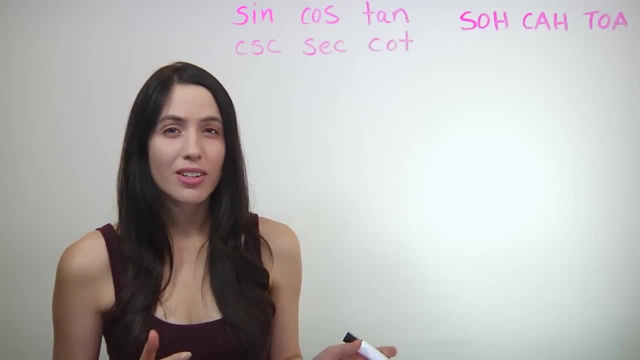 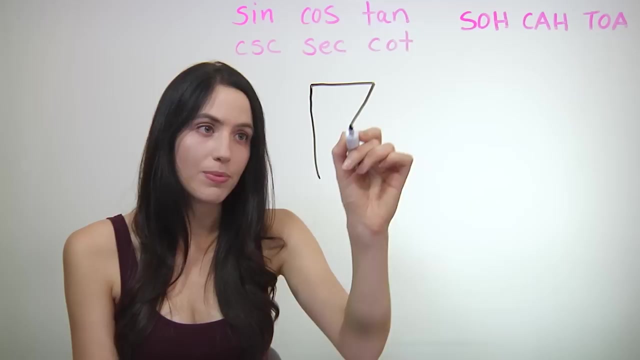 One thing that confuses people is when the right triangle is drawn at a different orientation, so if it's sideways or on its hypotenuse. So, for instance, you could have a triangle that's drawn like this, It's still a right triangle. 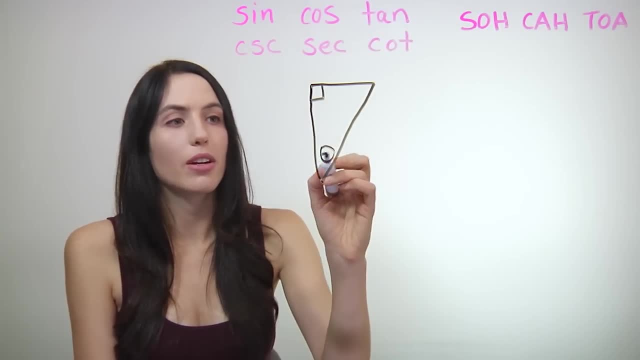 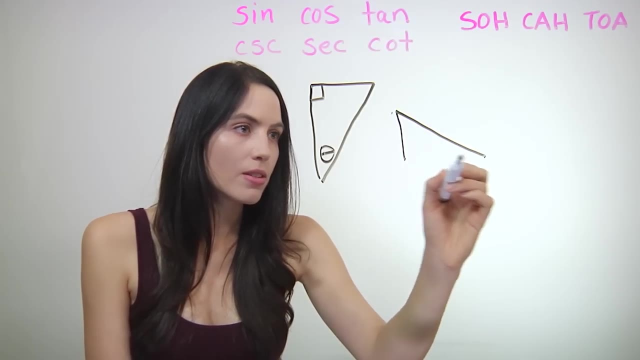 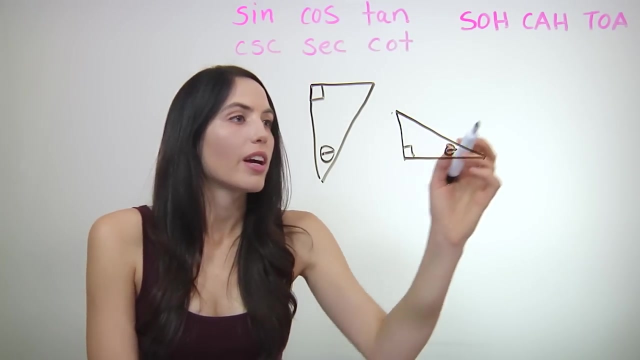 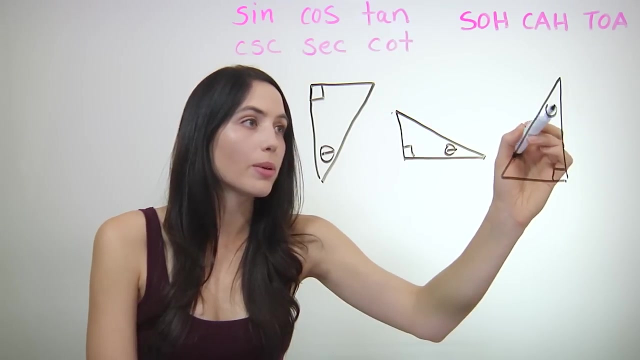 It looks kind of upside down. Your theta could be here. You could have a triangle that looks like this, So it's the reverse of the one in our example. You could have a triangle drawn with your theta up here instead of down here. 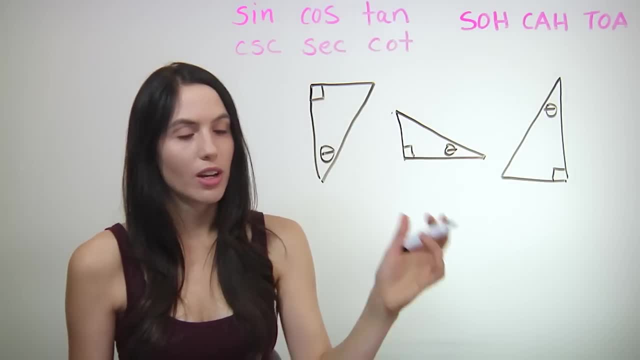 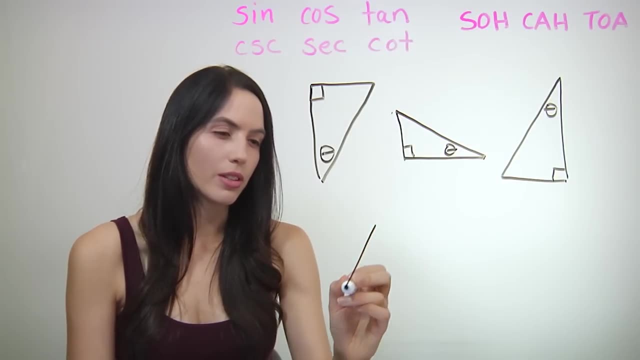 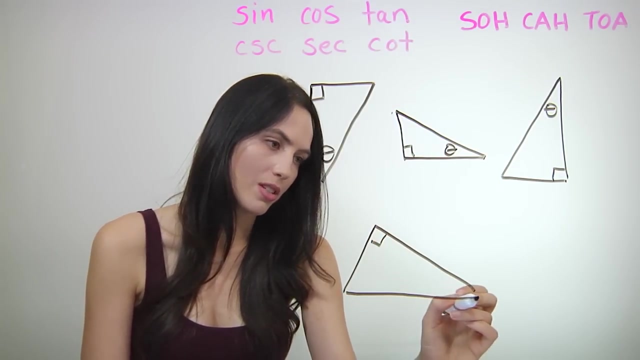 And the one that's most confusing to people is when the right triangle is drawn so that its hypotenuse is horizontal. It's sort of on the ground. So here's an example of that: If your right angle was actually up here, then your hypotenuse turned out to be horizontal. 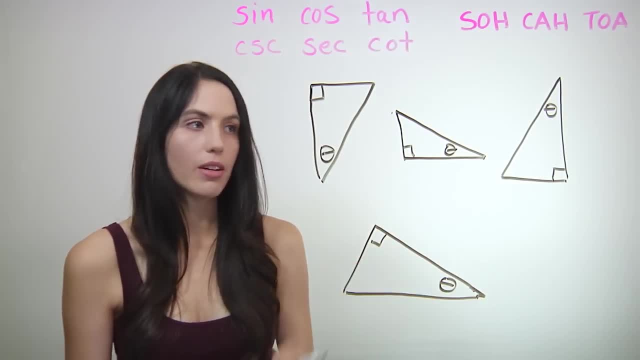 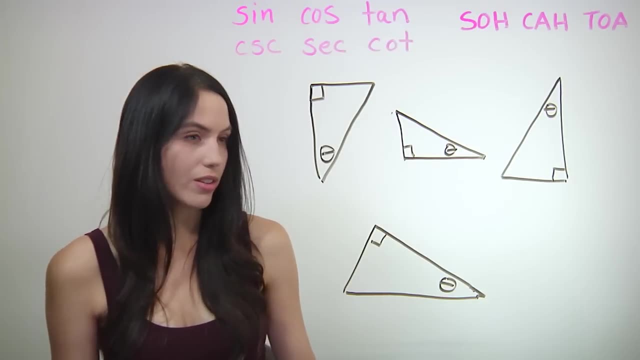 And your theta could be here or here. So let's look at these things and label where opposite, adjacent and hypotenuse are. for these triangles, In this example, in all of these triangles, actually, you can rely on your hypotenuse. 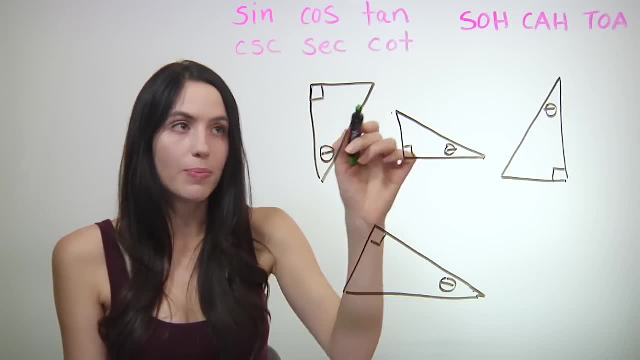 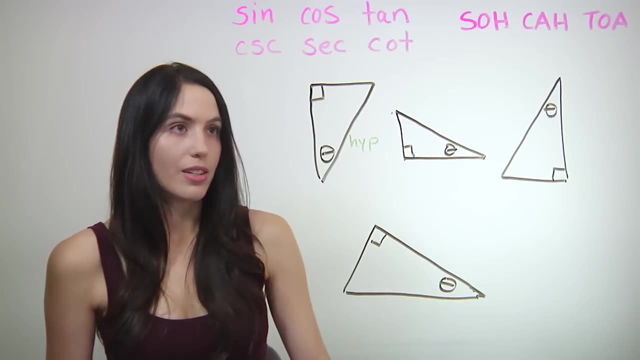 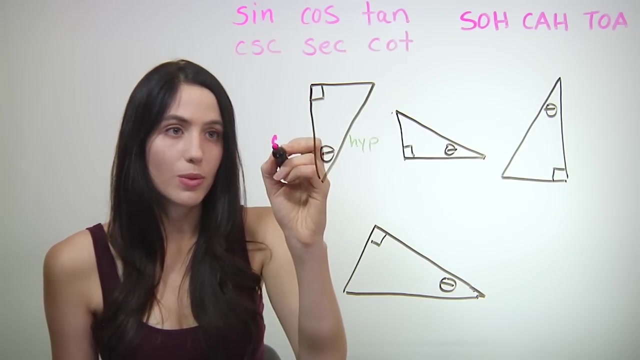 being the longest side. So in this triangle you can still tell that this is the longest side. so it would be your hypotenuse. The other side that's next to theta is still your adjacent, So this would be your adjacent. And then the other side that is opposite theta. 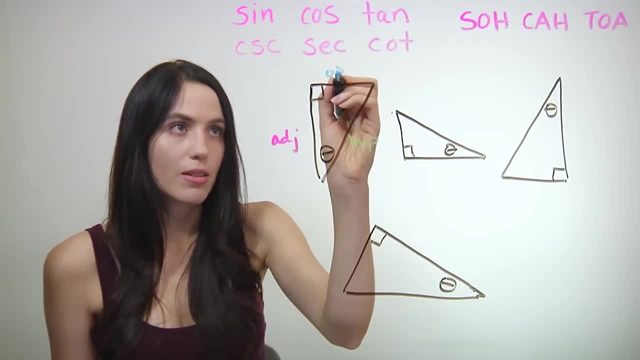 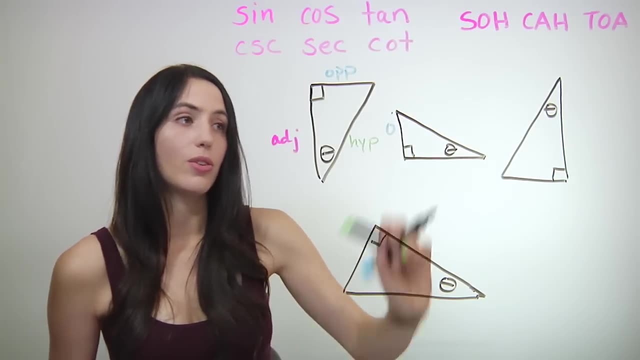 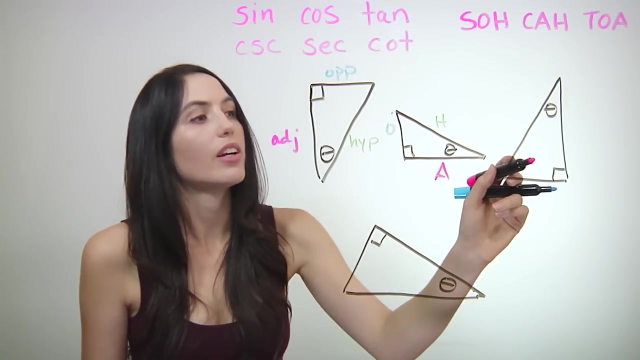 directly across from theta is opposite side. Let's label these as well. So across from theta is your opposite side, Longest side is your hypotenuse And the other side, next to theta, is your adjacent. Over here, your adjacent is this side. 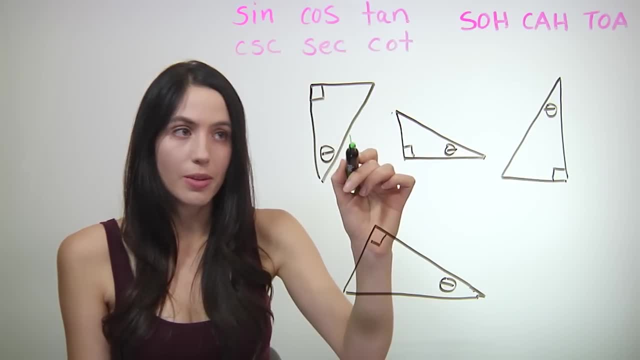 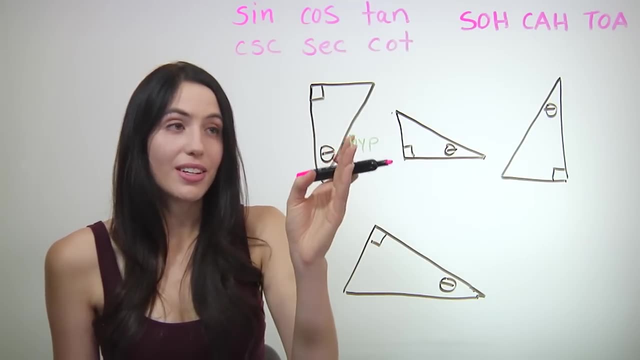 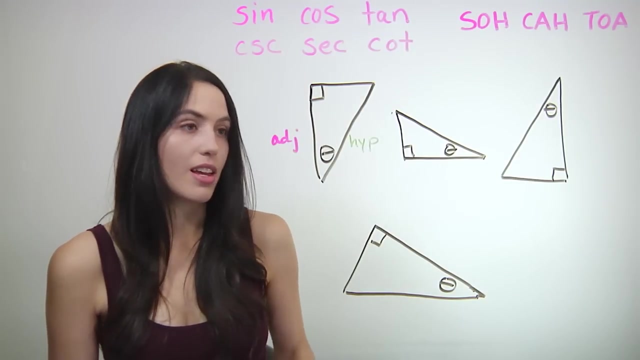 So in this triangle you can still tell that this is the longest side. So it would be your hypotenuse. The other side that's next to theta, is still your adjacent side, So this would be your adjacent. And then the other side that is opposite theta, directly across from theta, is opposite side. 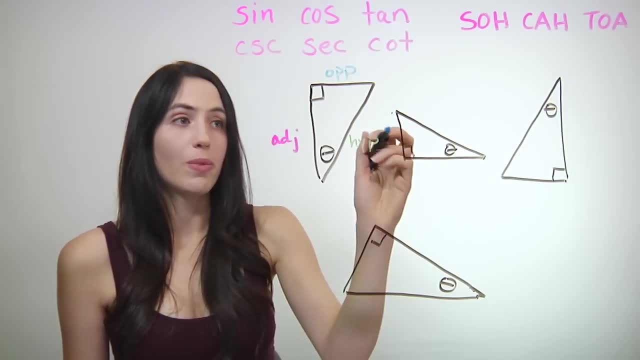 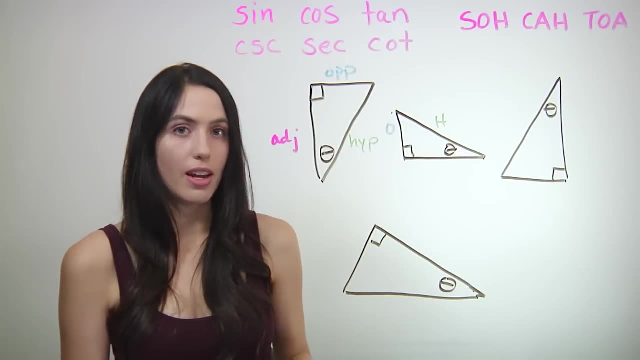 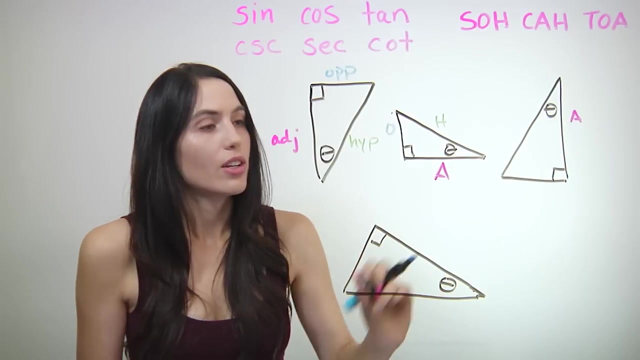 Let's label these as well. So across from theta is your opposite side, Longest side is your hypotenuse And the other side, next to theta, is your adjacent. Over here, your adjacent is this side. Your opposite is down here. 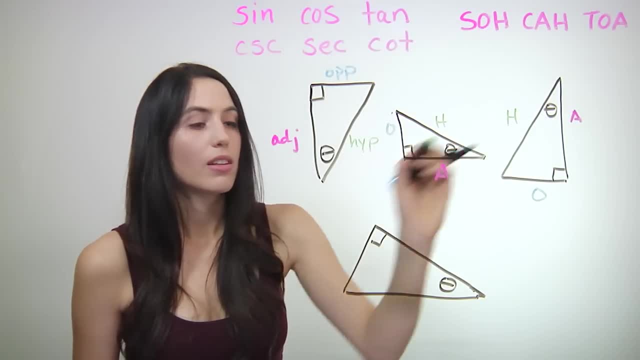 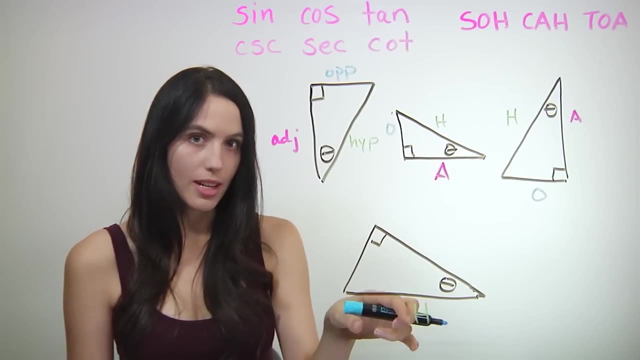 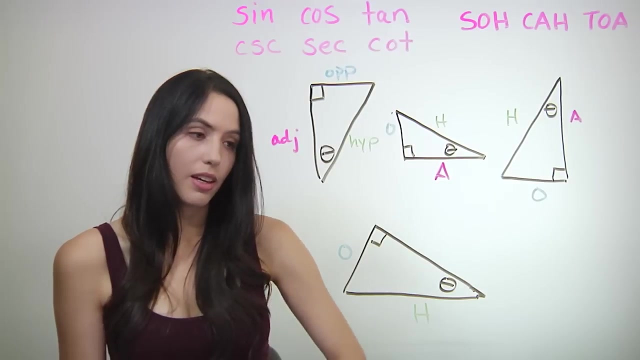 And your hypotenuse is the longest side. Okay, Down here longest side is still your hypotenuse, The one that's opposite the right angle, The one opposite theta is your opposite side And the other side, next to theta, is your adjacent. 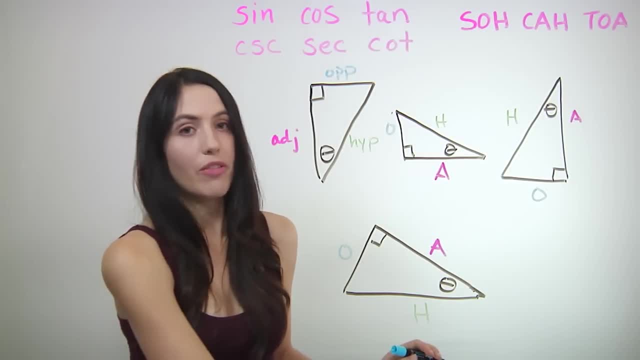 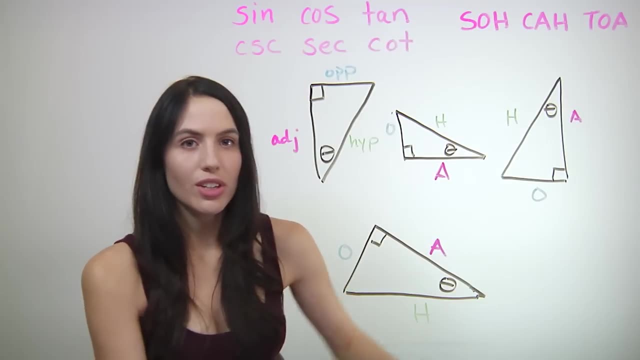 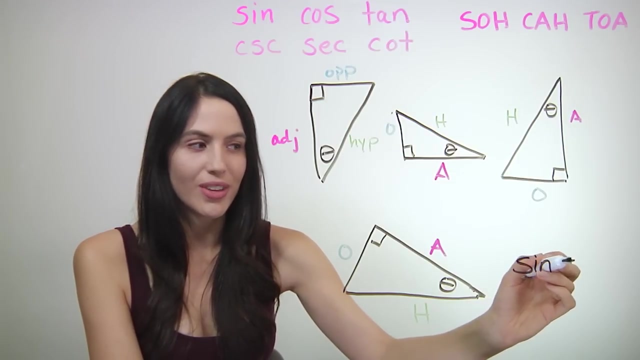 There's one more thing that trips people up in these problems: when you're finding the value of trig functions, When you write your final answer, make sure you put theta- You don't want to write something like this- that your sine equals 3 fifths. 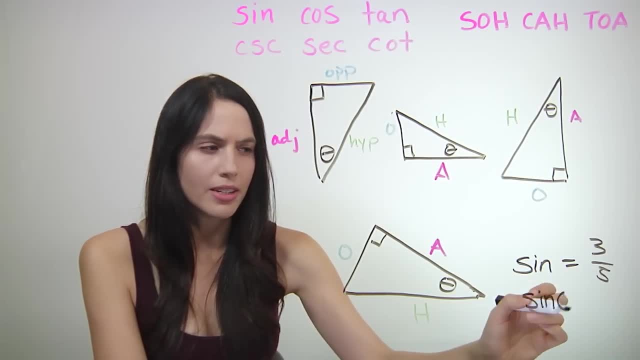 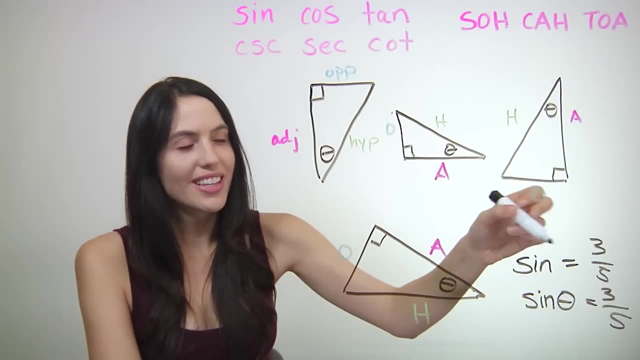 You want to write sine of an angle. Sine of theta equals a number. If you don't write the angle, this doesn't have any meaning. I know a lot of people forget it. I get it. I know It's a lot to remember. 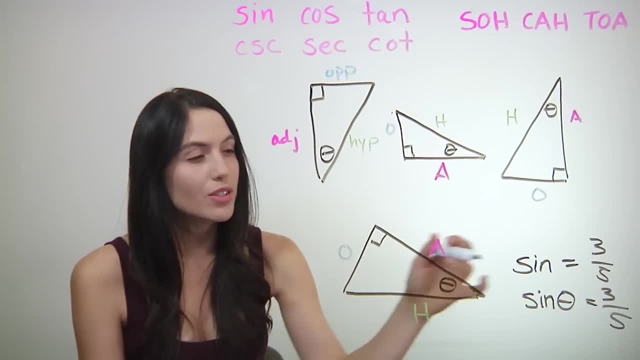 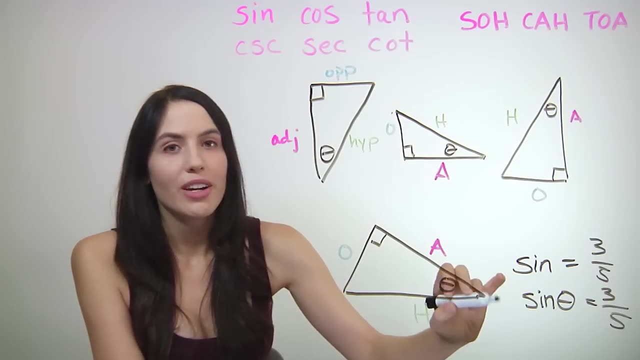 These trig functions are all new and weird, But if you don't write the angle it doesn't really make sense, It doesn't really have any meaning. So make sure you write your full answer as sine of an angle, cosine of theta, tangent of theta or tangent of x. 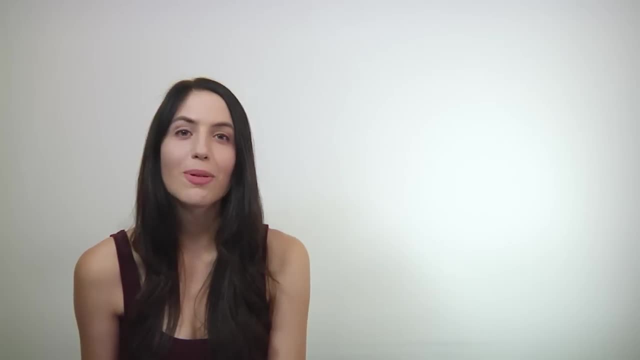 whatever your angle is called. I hope that helped you understand sines, cosines, tangents, cosecant, secant, cotangents. I know trig functions are super fun. It's okay You don't have to like math, but you can like my video. 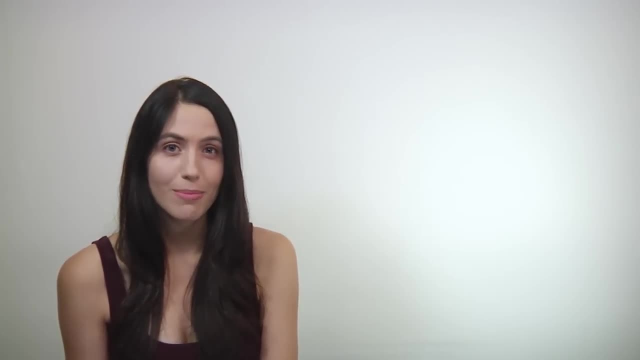 So if this helped you, please click like or subscribe below.